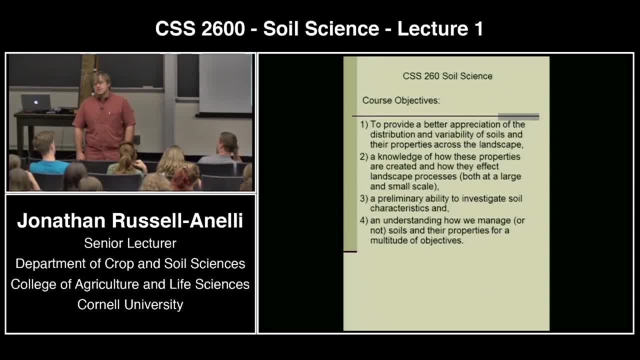 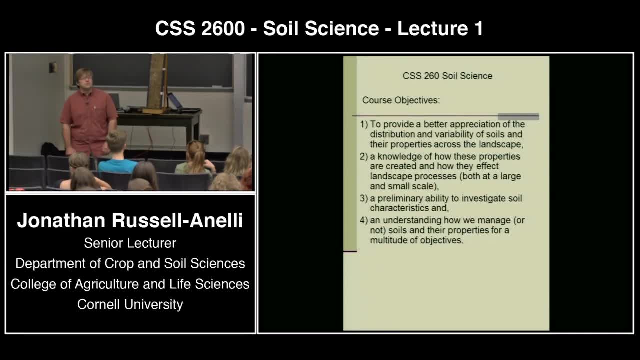 My name is Jonathan Russell-Linelli. I am the instructor for the class. I am a senior extension associate as well as a senior lecturer. I'm a faculty line but I'm not tenured. okay, I am the New York State something, something- soil scientist. Basically, I'm the liaison between the land grant. 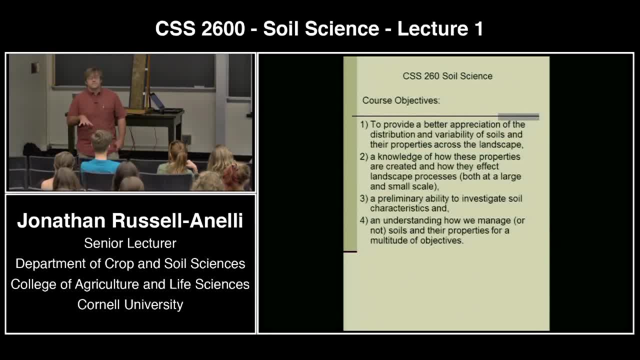 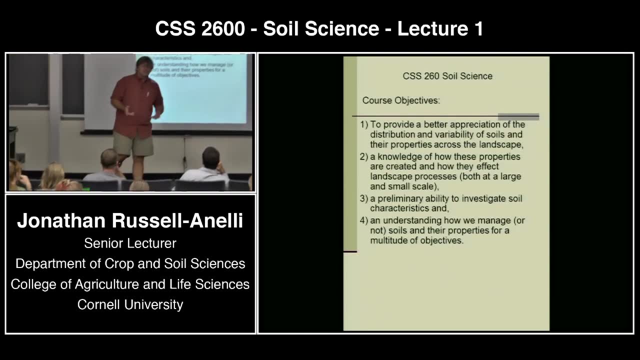 the federal government and New York State. when it comes to soils, I basically say, okay, it's good, That's basically all I do. I do a little bit more than that, But I really love soils. I came to Cornell as a grad student a long time ago, Then I left and I came back because they wanted me. 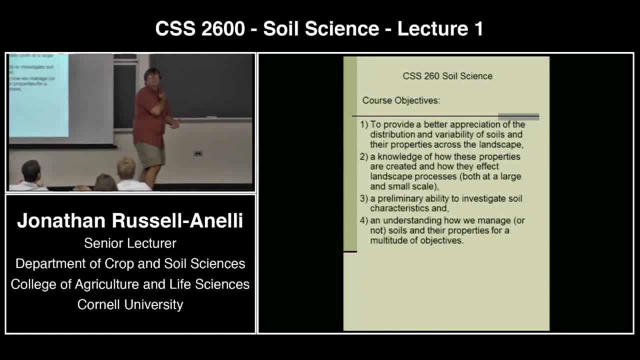 and I stayed ever, since. This is the longest time I've ever actually lived in one place. I've lived here nine years. I know that sounds like a short period of time, but it's actually pretty long for me. Ithaca, You guys are all upperclassmen at this point, and some of you as are transferers. I 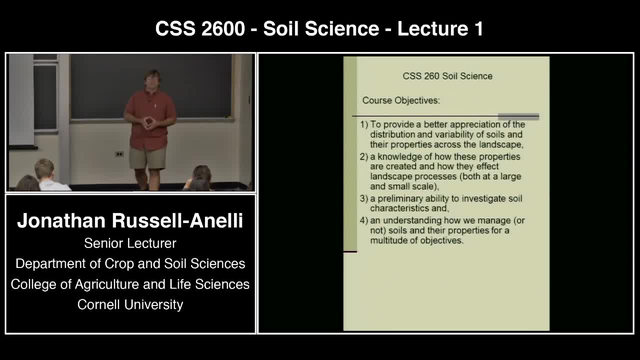 know that, But Ithaca is a really awesome place. You've had nice classes and you've had great time. awesome place. I hope you guys have a chance to explore beyond campus and you will certainly have an opportunity to do that with this class because there's 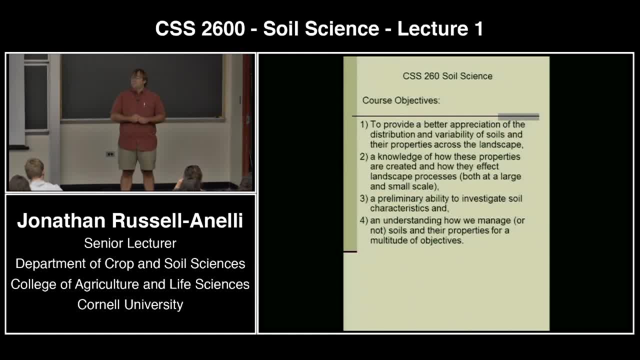 gonna be a lot of field trips. okay, I'm not gonna open up for questions at this point because I don't have a lot of information to talk about, but what I like to do is today is I'm gonna talk about the course objectives and I'm 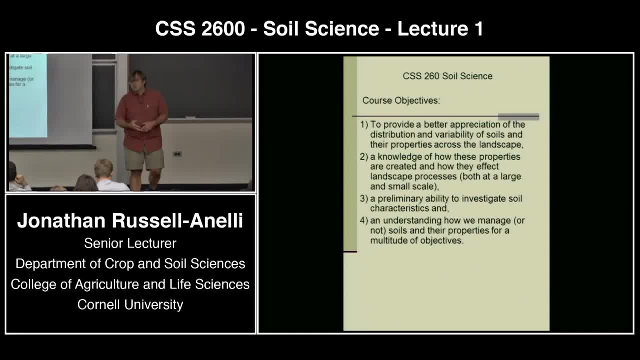 gonna talk about some logistics stuff. I'm gonna talk about the field stuff that we're gonna be doing, as well as the labs, some of the objectives of lecture as well as some of the objectives of lab course requirements, exam schedules, all that type of stuff, and then introduce you to us, introduce you to soils and 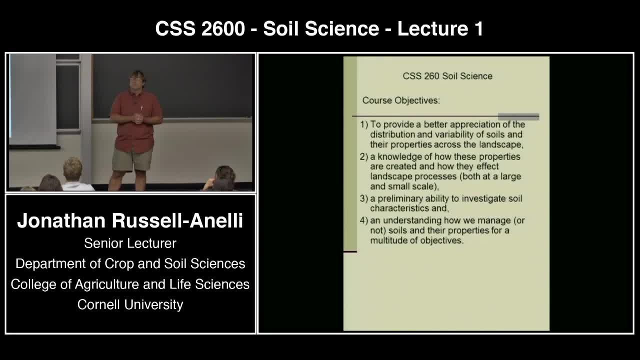 then I'm gonna tell you a story, and that's basically what we're gonna do today. all right, I also have- if we have time, we'll have a little exercise. I originally wrote that as homework and then I realized that was not what I should be writing. let's start with the right kind of language. okay, all right, so. 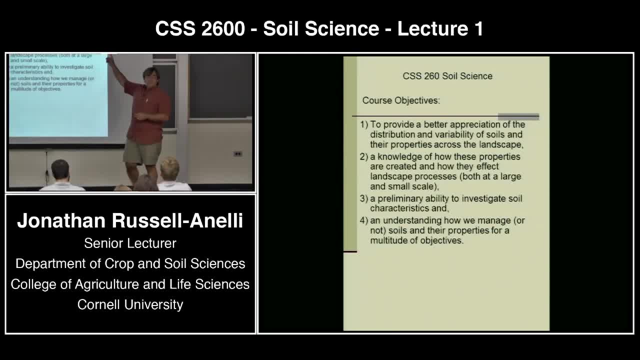 if you guys don't know what I'm talking about. I'm not gonna be talking about what you guys are in 2600, even though it's typoed up there as 2602 60, we have basically three course objectives. the first course objective is basically to 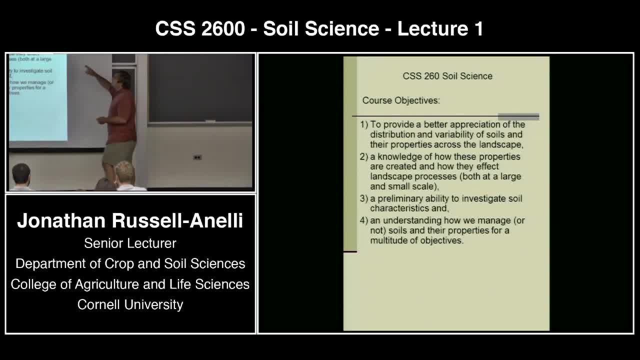 provide a better appreciation of the distribution and variability of soils and their properties across the landscape. this is introduction to soil science. the trial of the course is actually soil science. this course is a very, very large River, except it's about three inches deep. okay, we're gonna be. 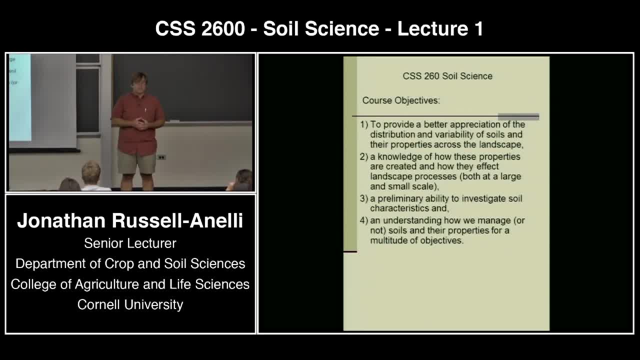 talking about a lot of different aspects of soil science, okay, but we're not gonna touch too deep on anything. but we want you guys to get an appreciation of what the nature of soils is, what the properties of soils is and how we interpret them. okay, the second objective is that interpretation, a knowledge of 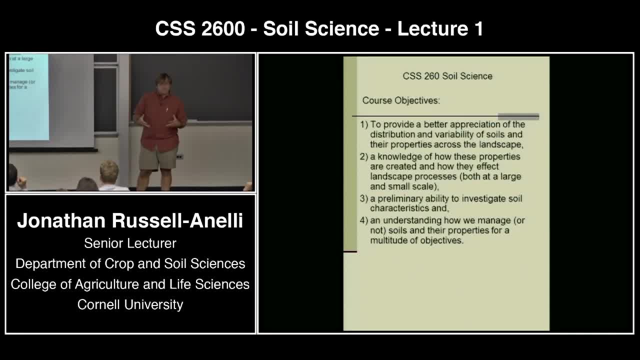 how these properties are created, what makes these soils okay, how they affect the landscape and the process of the landscape, both at the large scale and the small scale, and that's probably the last time you'll see me do large scale this way and small scale this way, okay, does anybody know what a large scale map is? 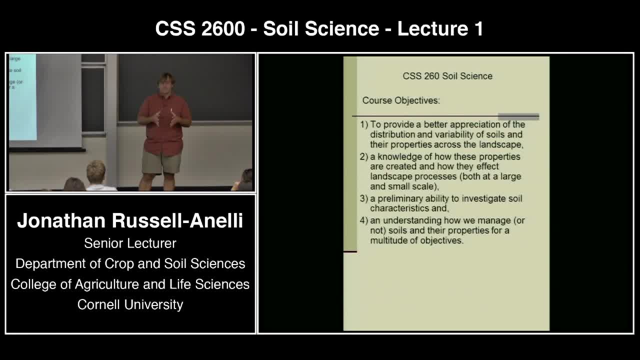 versus a small scale map. here's our first lesson of the day. has nothing to do with soils, has to do with math. terrible. large scale is one to one. it's big number one versus small scale, which is one to two hundred thousand. small fraction: okay, totally counterintuitive. but just so you know that's what we're talking about. 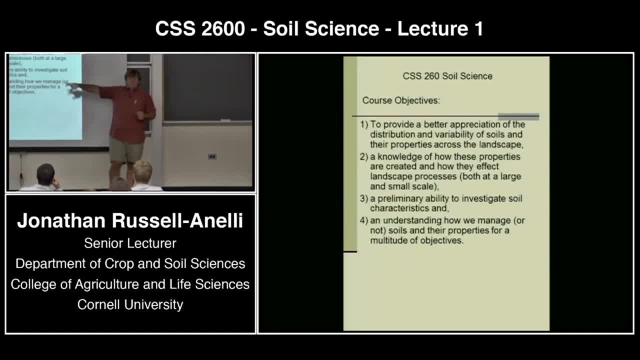 okay, the next thing that we're going to be teaching you guys do is gonna be a lot of tool use today and not today. this whole semester we're basically gonna be teaching you guys a preliminary ability to investigate these soil characteristics. so a lot of tools, a lot of technique type of stuff and finally, 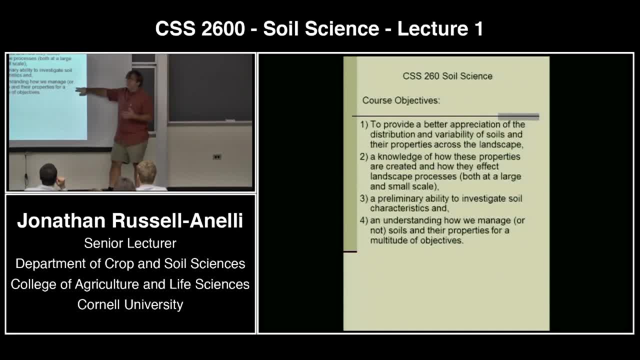 which I think most of you are really more excited about, maybe, hopefully- is an understanding of how we manage these properties, how we manage these soils for a multitude of different objectives, whether you're an engineer, a farmer, a homeowner, a road builder- lots of different uses for these soils, okay. 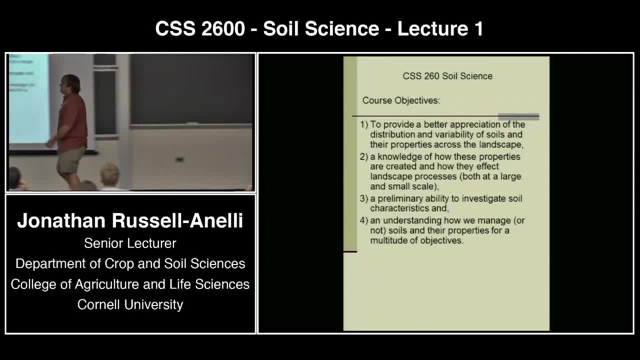 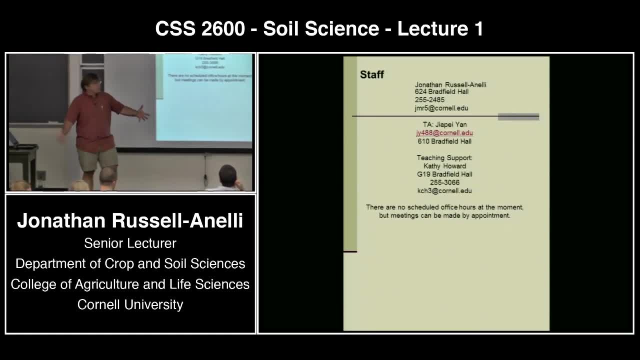 make sense. okay, staff: I've sort of introduced myself already: Jonathan, Russell and Ellie. okay, my office is not actually 624 anymore, it's actually 1023. okay, I just moved offices and I forgot to change that email is the same email and the phone number is the same phone number. okay, if 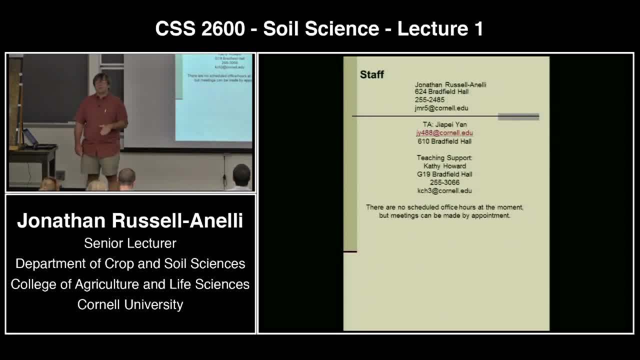 you have any issues, get in contact with me right away. this has actually already come up. somebody's gonna have to miss Friday's lecture. Friday's lecture- that's not a big deal in the grand scheme of things. it is a big deal if I don't know it ahead of time. okay, if you have a wedding to go to your cat. 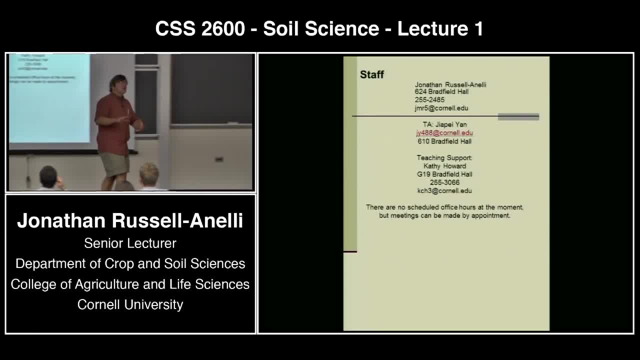 died. god forbid, your cat died. you've got a game that you have to go to. okay, tell me ahead of time, don't tell me after the fact. okay, all right, TA Jaipei is here. Jaipei Yan Jaipei is in the department she is in. Elena- I can't pronounce her last name- that. 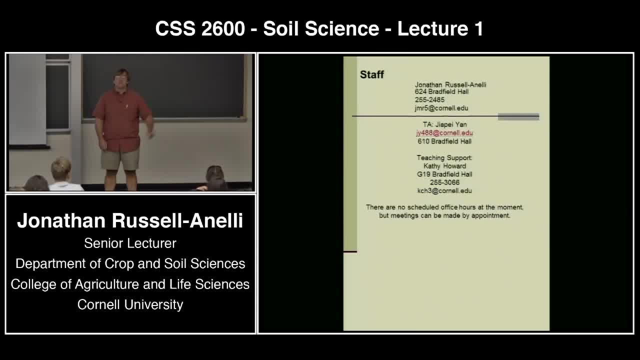 Dementic last. she is one of the soil ecologists in the department. Jaipei did this TA ship last year. she's a pro at the department. she's a pro at the department. Jaipei did this TA ship last year. she's a pro at the. 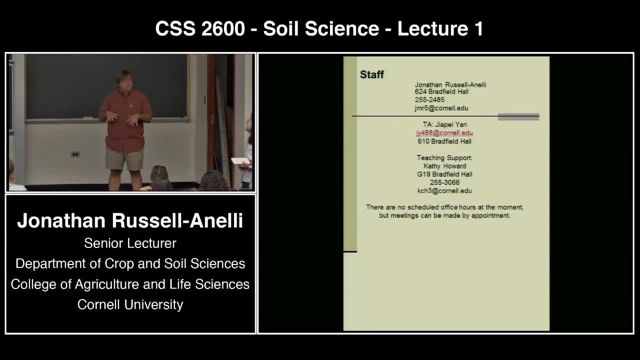 this at this point. if you have any issues that you can't get in contact with me, Jaipei is the person, okay, and her office numbers up there fix that, okay. the last person that you guys should meet for right now is Kathy Howard. Kathy is the red shirt back over there. red shirt, not. 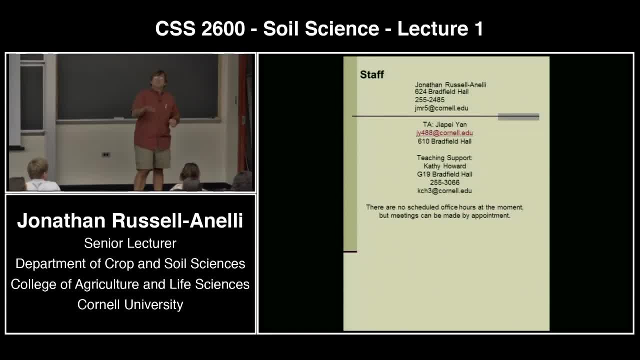 in the Star Trek sense of the word. okay, she is that tight, totally missed everybody okay. okay, she is a teaching support specialist. she is basically the person that makes sure all of our logistical kind of things happen. okay, she will be with us on a number of the field trips and she will. 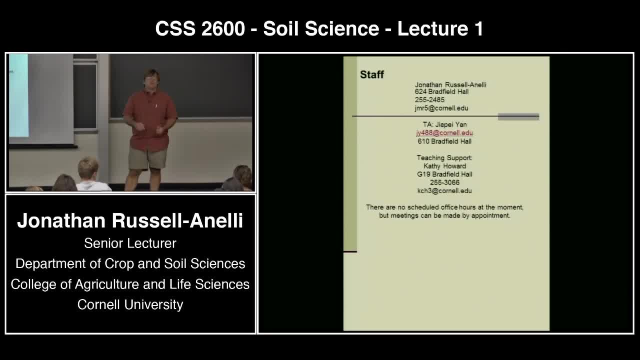 be with us on a number of the labs and you'll see her in and out all the time. if you have any questions about anything, ask Kathy as well. okay, all right, at this point at this moment there are no scheduled office hours. there's 82 of you. 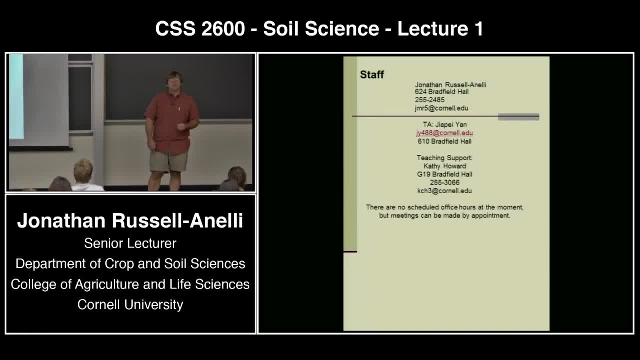 or something like that. we'll see what happens in the next couple weeks. there's a lot of you. I'm not going to schedule office hours. my teaching schedule this semester every fall is really tight. I basically have two mornings off and lunch times. okay, if you have an issue, email me. we'll schedule some time to. 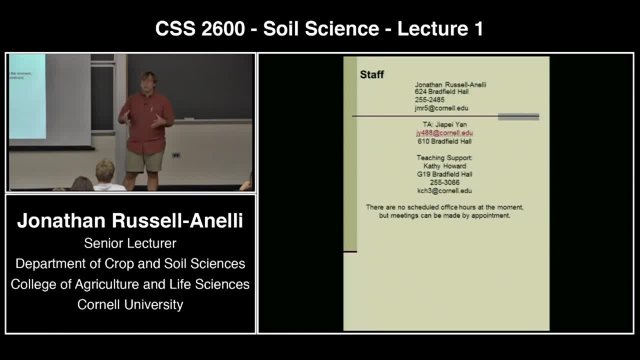 come in and out so you guys can talk. okay, we will schedule the time. I will make the time for you guys, okay, so meetings can be made by appointment. that also applies as I pay and Kathy. okay, but I'll be the first person you hit shot. I pay a second, Kathy third. okay, unless it's an issue with me and then go. 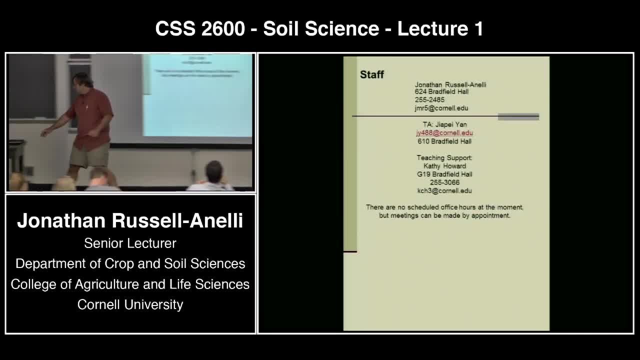 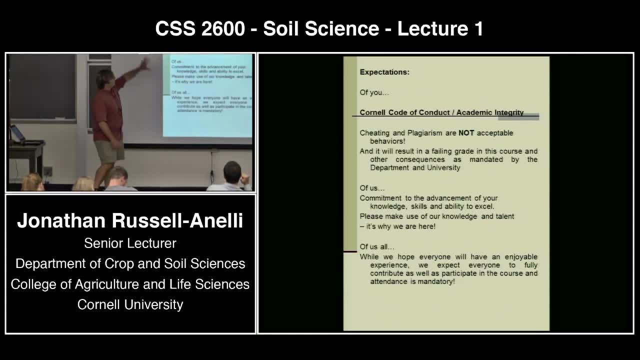 straight to shape a: okay expectations. this is the bad part. good part of the class, bad part of the class is down right in the beginning, there. expectations cheating and plagiarism is not acceptable. what can I say? it's not acceptable. if you do it, we will catch you and you will go straight to the 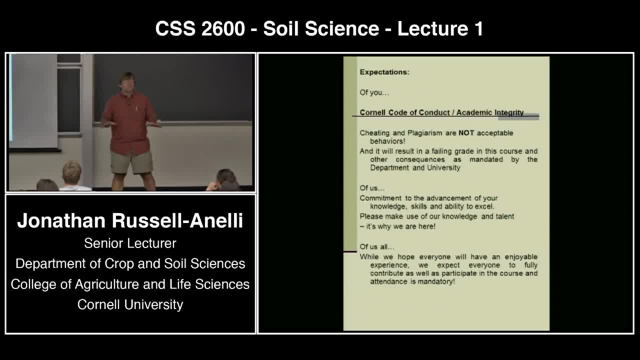 chair and the Dean. I'm not dealing with it. it's happened in the past. I am NOT dealing with it. you guys shouldn't have to deal with it either. okay, don't do it. this is a class that you don't need to do it. okay, now, just to give you one little more piece of why you shouldn't do it. 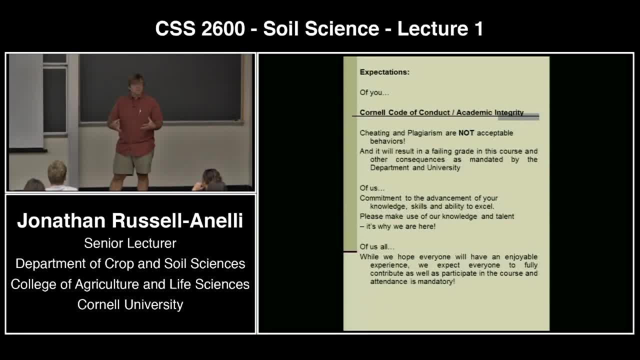 basically all of your submissions, any kind of academic thing that you were handing in to us, is going to be electronic. we're basically going to run it through the screener, okay, so just don't do it, okay, okay, yeah, all right, cool, all right. but I will say to you from our point, this is the better part of it. we are 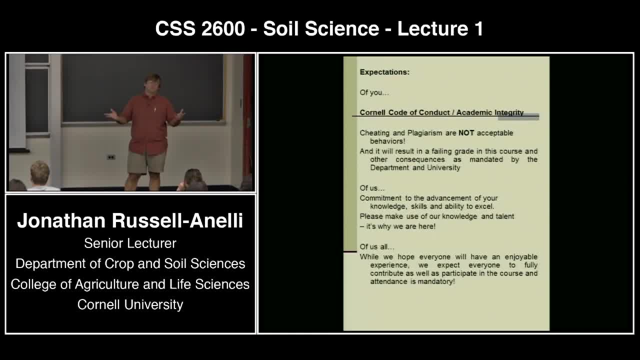 really committed this class. this is an awesome class. we think it's an awesome class. it's up to you to judge, but we think it's an awesome class. we love soils, we like being here. we really want you guys to appreciate these soils. and I haven't looked at everybody's major at this point, but the majors that I've seen. 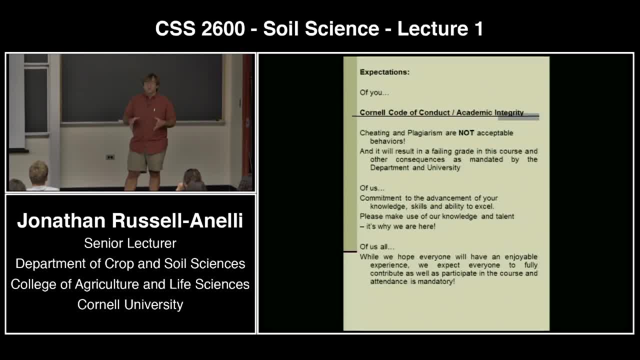 that you guys are associated with soils is very important to you, whether you know it or not. okay, and I'm hoping at this point you probably do know it already. okay, soils are really cool and we want you guys to have the skills and the knowledge and the ability to be able to take advantage of that. okay, of all of. 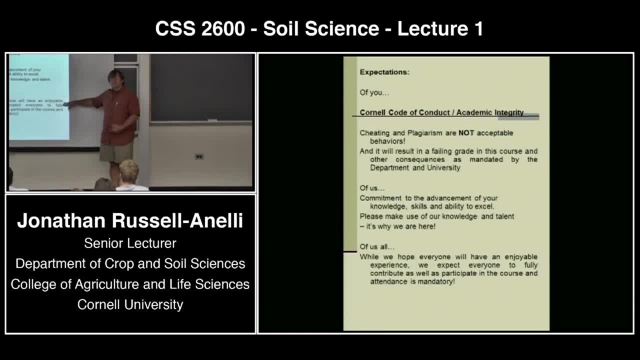 us, while we hope everybody. so I changed this. I said this yesterday. this is a good time, at which point I realized I'm not supposed to say that anymore, so I hope you all have an enjoyable experience. okay, we want you to have an enjoyable experience. okay, we expect everyone to fully contribute, as well as. 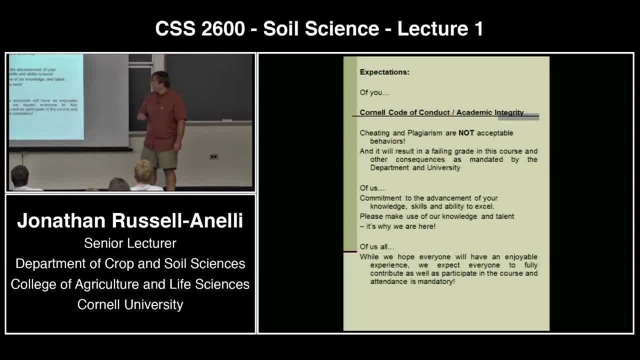 participate in this course. okay, and in life I will say: attendance is mandatory, both in the- certainly in the labs and, hopefully, in lectures. I'll see you all the time. I understand that accidents occur and things arise. okay, I will not be taking attendance. uh-huh, I won't be taking attendance, but there will be. 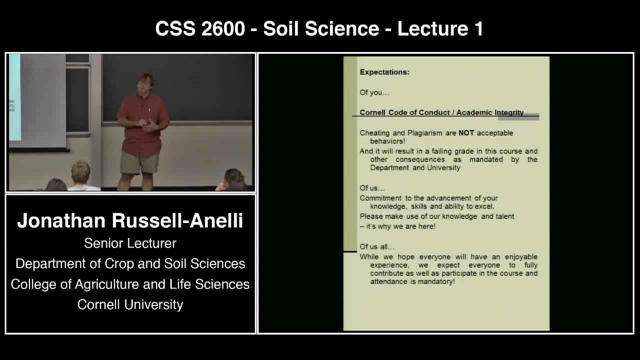 activities in class that you will have to do, that your name will be attached to. okay, things happen. you had a bender the night before, god forbid, the cat died, whatever. okay, please come to class. I know it's nine o'clock and Monday is a tough one, but today's 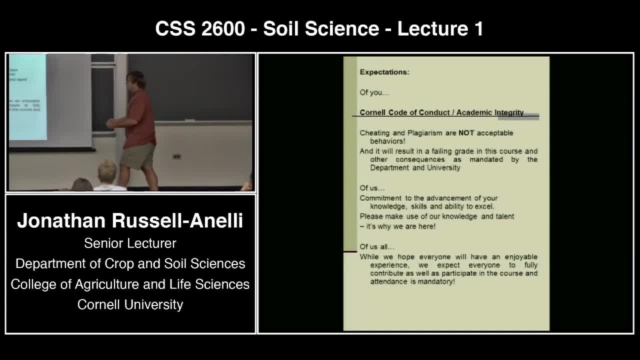 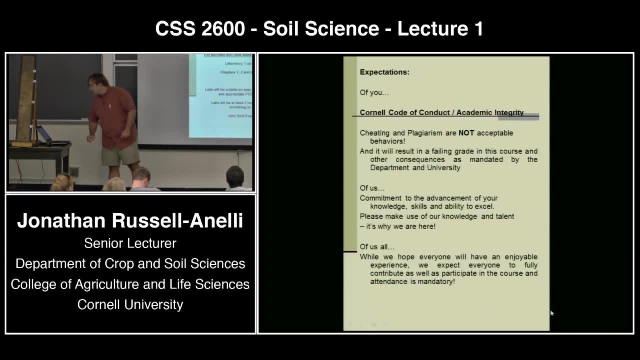 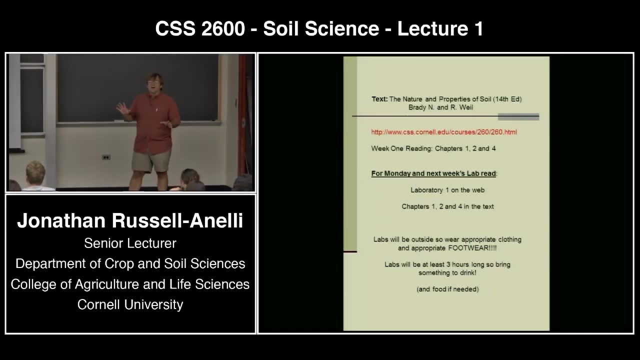 Wednesday. you're all here, right, you can do it again. okay, cool, maybe not. there we go the text. has anybody had got the text yet yet? yet has everybody got it? anybody's got it? somebody not have it? that's okay. 14th edition. it's the older version. I hold off until the very last minute before they force. 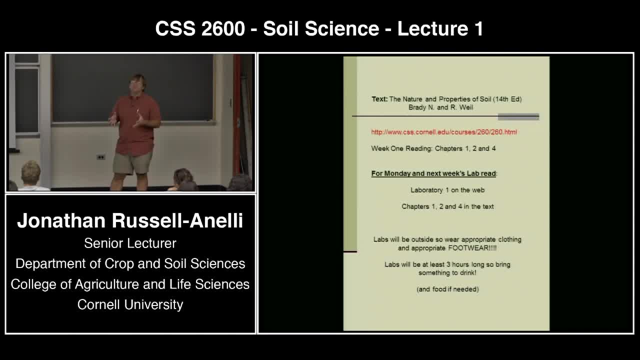 me to get the new edition, so there should be a lot of used books out there. okay, get it. it's a good book. it actually sells back fairly well too. it's an advanced book, but it's written at the level of an introductory book, so there's. 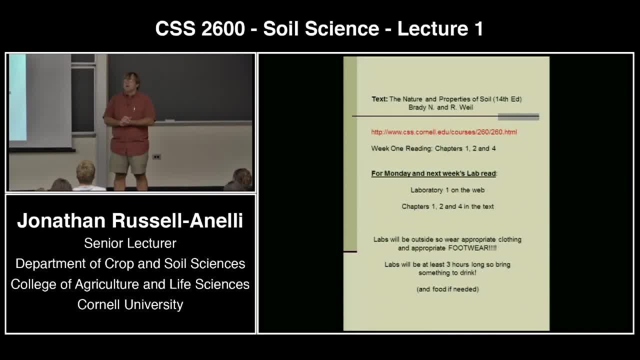 a lot of really good stuff in there that we probably won't be touching on this semester, but all the stuff that we're touching on is actually real well written. okay, it is a. the nature and properties of soil by Brady and Whyle. okay, its fourteenth-edition. 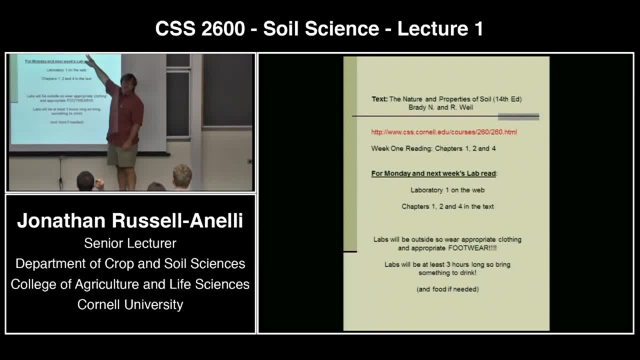 we actually have readings for the beginning of this. the tail end of this week, in the beginning next week, which is chapter, is one, two and four. okay, four Monday and next week's lab. I really want you guys to be reading this, okay, which also brings into point: 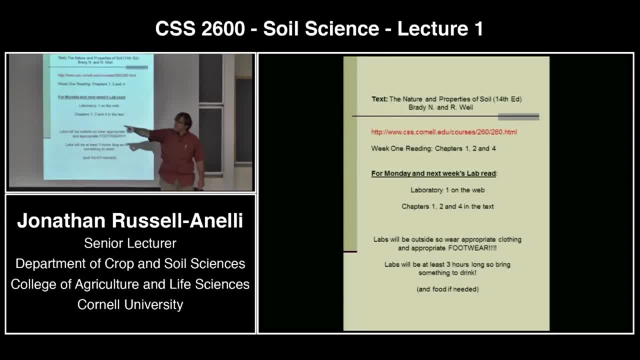 that we have a webpage. okay, the web page i've written over there so you don't have to scramble. okay, we are not on blackboard. I don't like blackboard. It's my fault, I apologize. We have our own website, Basically, logistically, information-wise. 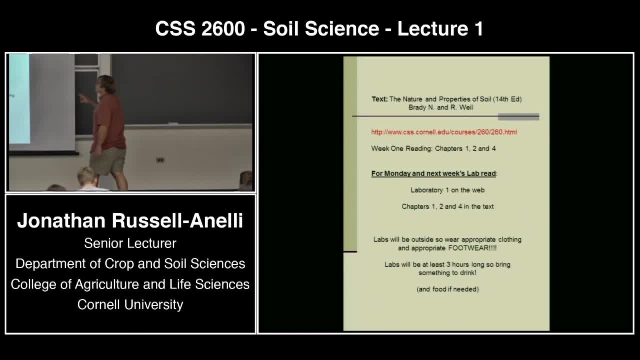 everything is on the website. So go to the website, get yourself familiar with it. It has basically five sections. The first section is the home, which basically is sort of the introduction. The second section is the lecture section And in the lecture section, every lecture. 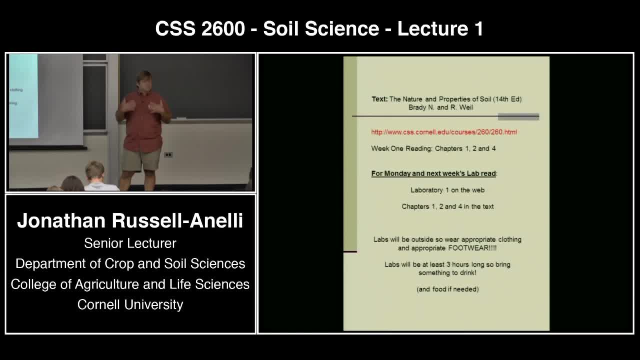 there's a PDF for it So that you can download that, make a copy, put it four slides per page or whatever. I don't want you guys to waste your time drawing the pictures that I've drawn on the PowerPoints. Spend your time listening to what I'm saying. 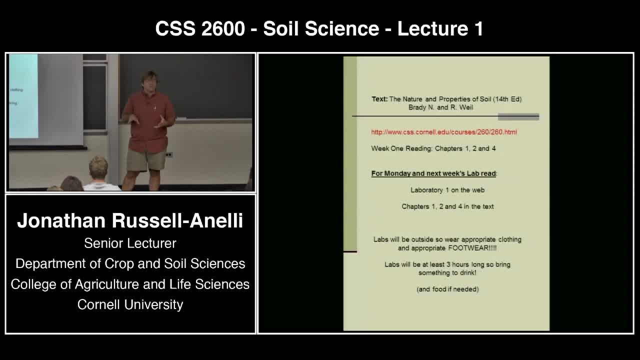 taking notes from what I'm saying, taking notes of our discussions, because we will be having discussions. Don't waste your time drawing what I've got on the board. There is also. the next section is the laboratory section. All the laboratories for the entire semester are online. 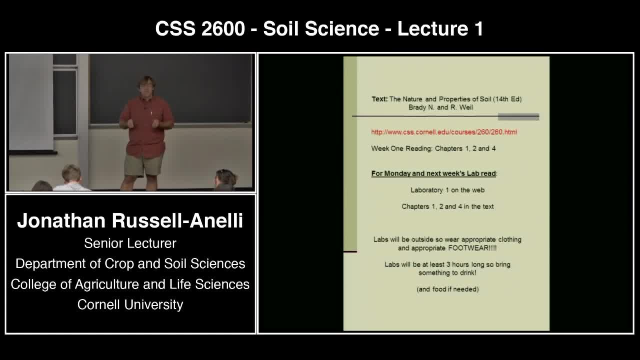 I do expect you guys to have those copied and read by the time you come to lab. You don't necessarily have to bring the copies of the lecture notes, because you can keep that on your computer or whatever. That's fine. But I do expect you to have a hard copy of the lab notes. 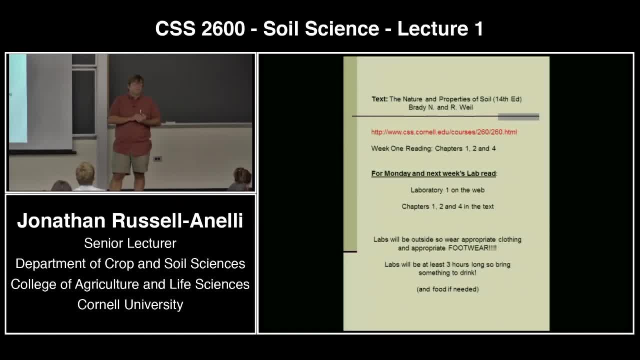 when we go into the field. It's hard to take the computer into the field. OK, labs will be outside, So I expect you to wear appropriate clothing, But, more importantly, I expect you to wear appropriate shoes. I really don't care if you come in a gold LeMay evening dress. 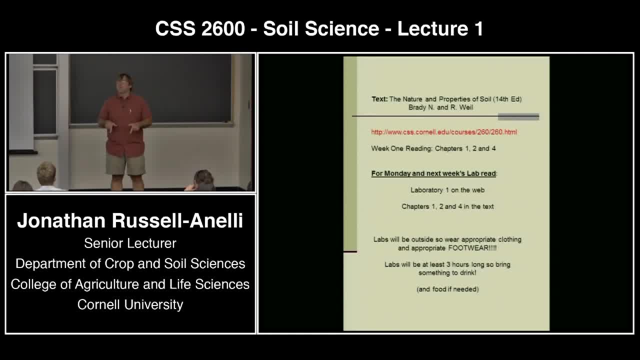 But you will be wearing army boots or something appropriate, ie closed-toed shoes, No flip-flops, No sandals that don't have toes that are closed, No high heels. I have had them all. I do not want them. 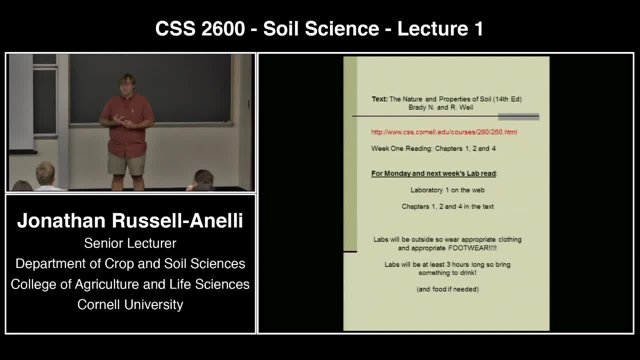 You will not be getting on the vans if I see those on your feet. Also, when we are in the lab, there's glassware, Things get broken, There's needles. There's all kinds of stuff in the labs. I don't want inappropriate footwear. 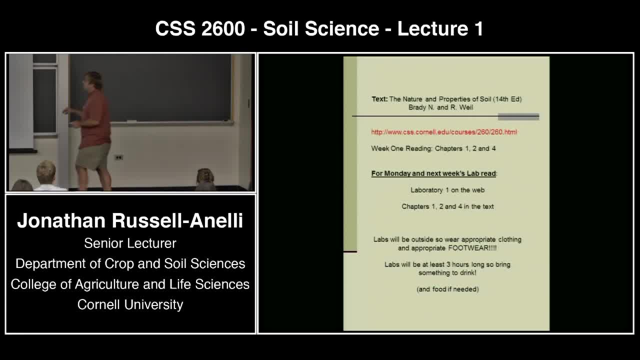 That's my fetish for the day. All right labs will be at least three hours long, So be prepared, Bring something to drink And, if you need, bring food as well. The lab TAs will love you for it. Now I will too, because I don't have to listen to. 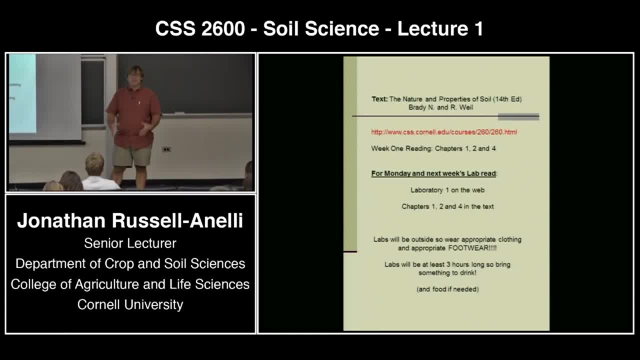 I have two kids at home that they get thirsty all the time. We have like a gallon of water. I have a gallon of water in the back of the van and that still doesn't help. Okay, Please bring water Grades. 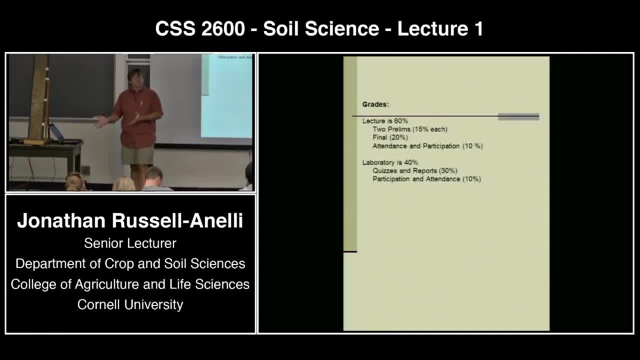 The grades are basically broken up into two components. One is the lecture component and one is the lab component. Can you guys all see that? Hopefully that's big enough. The lecture is basically 60% of your grade and it's based on three prelims or two prelims. 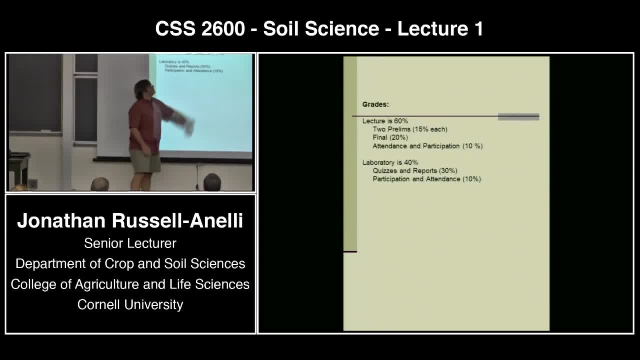 and a final, as well as attendance and participation. The two prelims are worth 15 points each. All right, The final is worth 20, and then attendance and participation is 10%. Okay, It's going to be harder to do participation here, but it won't be that hard to do attendance. 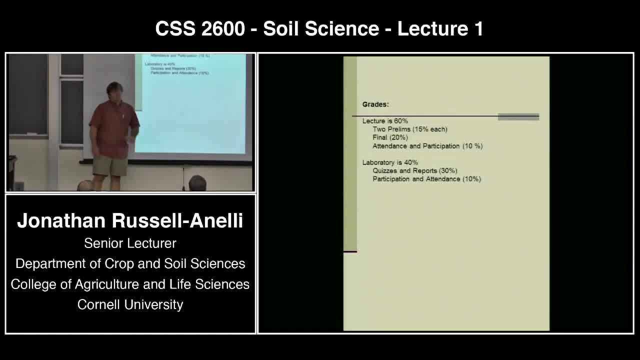 Okay, The lecture or the laboratory. there are quizzes and reports that are associated with the labs. Okay, There are going to be, I think, 12 labs total. Eight of them are basically outside labs or somewhat outside. Okay. 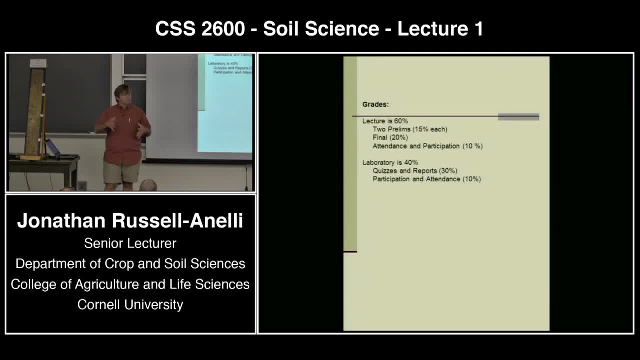 Not all the labs have a report attached to it, and some of the labs are multiple labs. Okay, All right. So there's a series of events that happen over a couple of days- or a couple of weeks, I should say- and there'll be one report at the end of it. 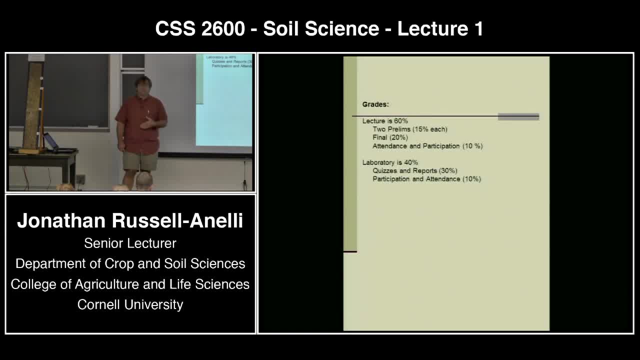 Okay, But there are reports and quizzes associated with those. Okay, You will also notice that participation and attendance is 10% here, so basically, 20% of your grade is showing up and opening your mouth every once in a while. Cool deal, huh. 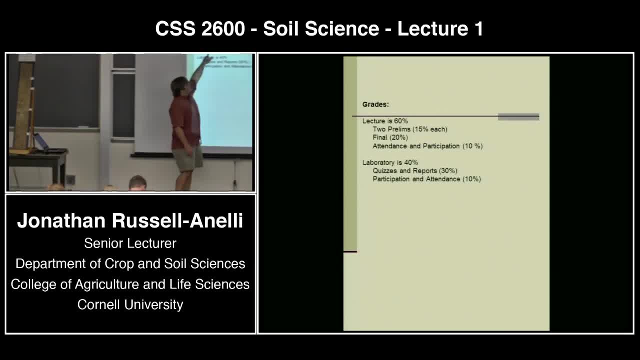 Okay, But you will note that this is attendance and then participation, and this is participation and then attendance. If you don't show up, you've already lost. Okay, We do expect you to participate in these labs, Ask questions, Support your fellow students. 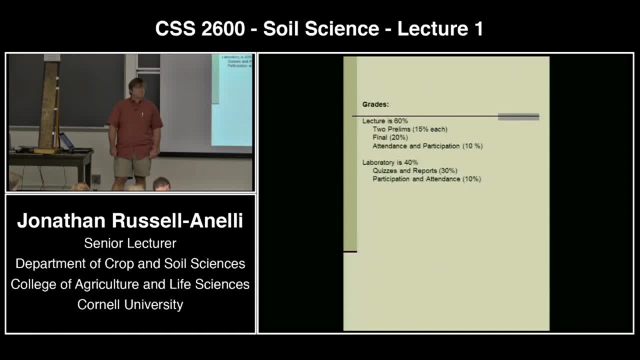 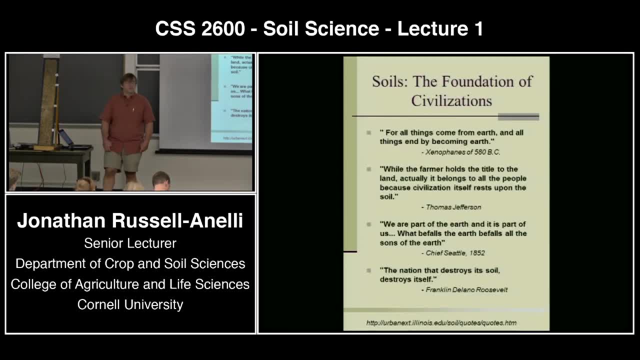 Do things. There's a lot of stuff that you guys are going to be doing. Okay Questions so far? No. All right, We've gotten through the hard part. Let's start introducing you guys to soils. I've got a couple of quotes up there. 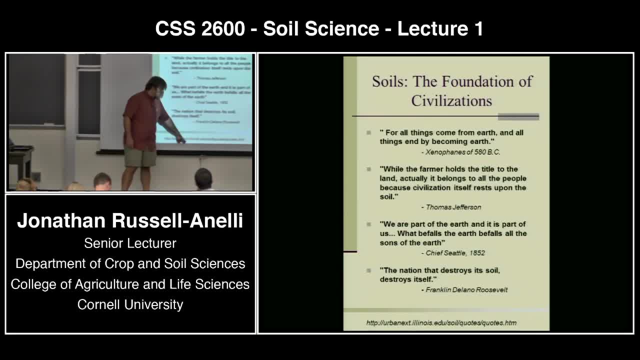 There's a whole boatload of quotes. If you really want to have some great quotes, go to this website down here. I've got a couple of quotes up there. I'll write it down later if you want it. But basically we're going to be talking about soils. 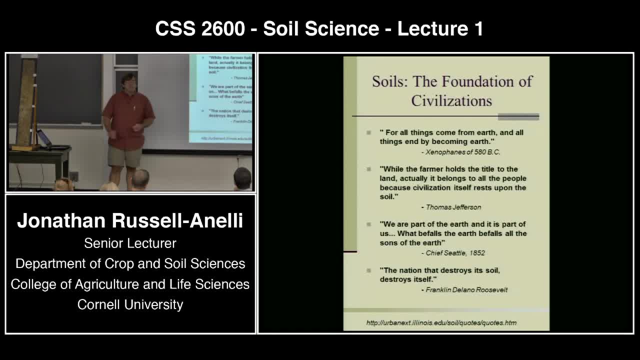 No big surprise there, But coming from a lot of different people and from a lot of different perspectives and a lot of different eras, soils have been felt or considered to be pretty darn important. Okay, Now, that's not my plug to say you should be in this class, but it's my plug to say hey. 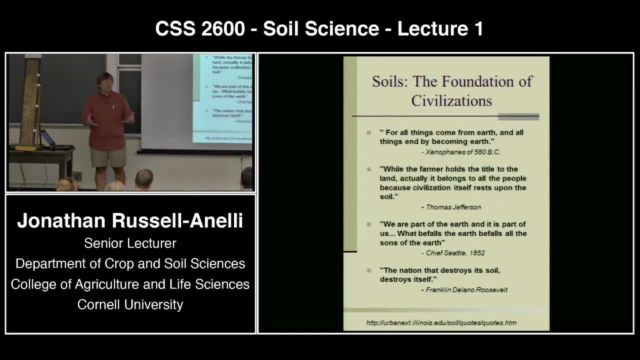 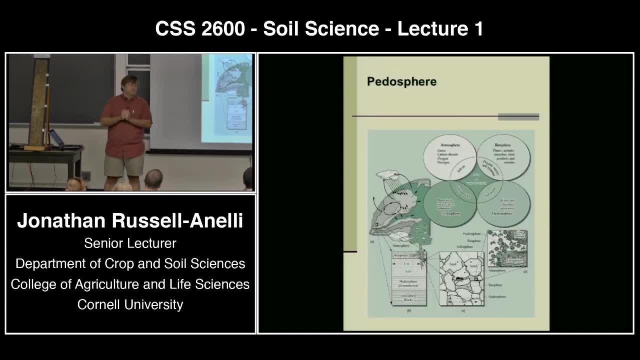 we're not the only people that recognize that this is important. So let's talk about what soil is. I suspect that a lot of you guys came into this class with some expectation of what soil. is Anybody willing to contribute at this point, or share at this point, or is it still too? 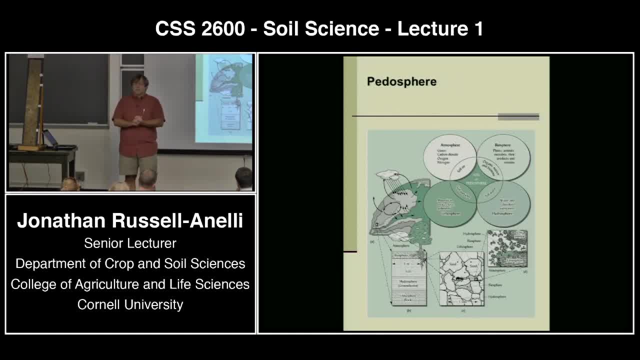 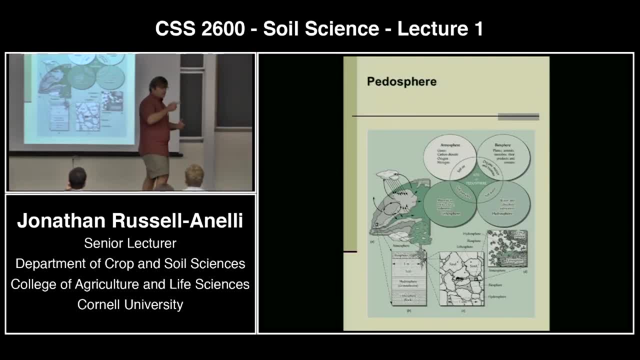 early in the semester to say anything, or early in the day. What do you think soil is? Any ideas Go Dirt, Dirt. Actually, technically dirt is not what soil is, but you're pretty much on the ball- Dirt. 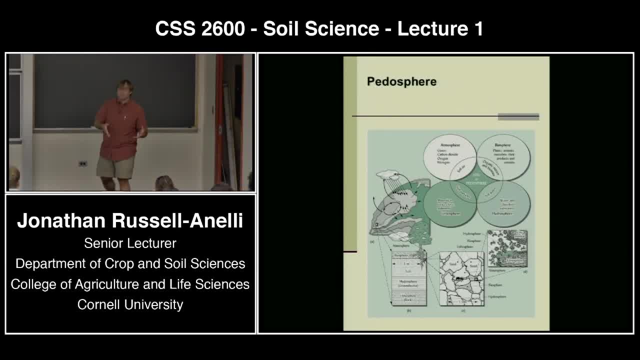 Okay, What do you think dirt is? Dirt is a technical term, Not that anybody would know it. Dirt is soil that is out of place. You've dug up something. You've moved it. It's now dirt, But prior to moving it it was soil. 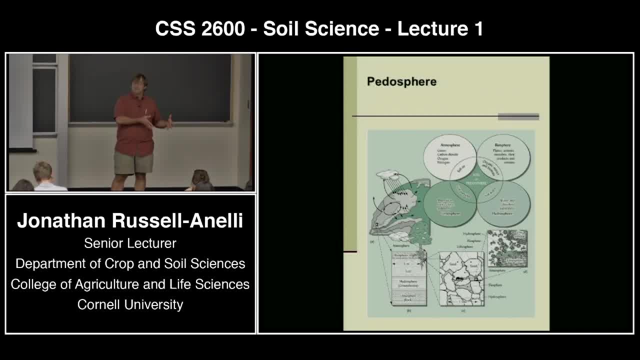 That dirt, given time, will become soil again. Okay, Any other ideas? What do you think of soil? What do you think dirt is Dirt soil. What do you think it is Go? Minerals and organic matter. Minerals and organic matter. 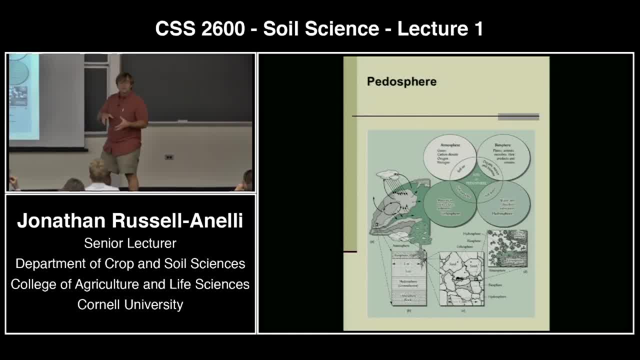 So you're getting into what it's made up of. That's a good way, and that's one of the things that we're going to be talking about today. What is the material of which soil is made up? Basically the same thing as dirt. 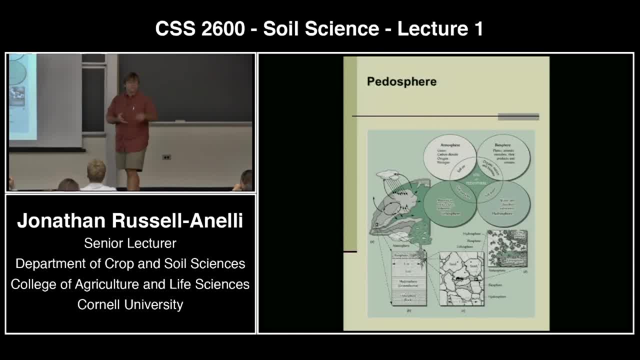 Mineral material, organic material, Anything else. Any other ideas Go? Microorganisms. Microorganisms, Living organisms, Things that are in the soil, that use it as an environment. Okay, We know that the living part of this material is also what we consider soil. 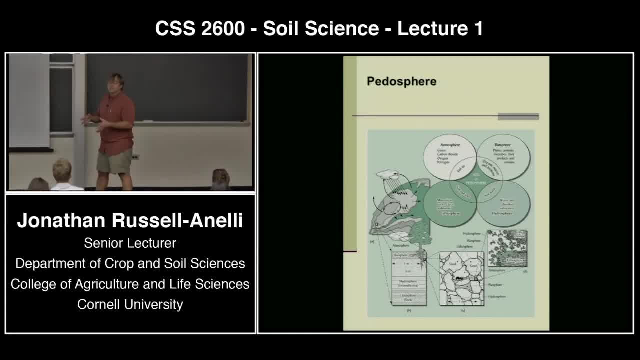 It's not just the dead stuff. Okay, Any other ideas Go? Water and air. Water and air- Ah, that's a good one. Generally people don't think of those, but they often think of it as a source of it. 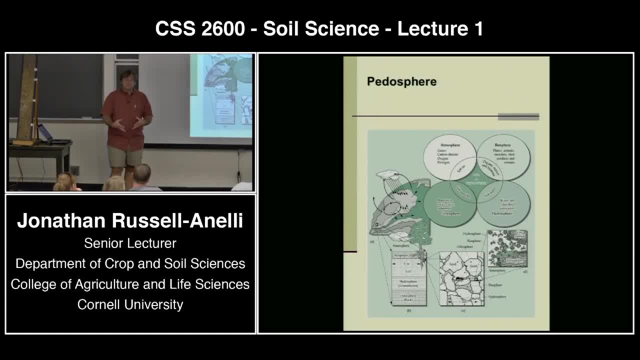 Generally, most people, when they think of soil or dirt, they think of a thing, Some kind of hard thing I can touch. I want you guys to think of soil from a different perspective. I don't want you to think of soil as a thing. 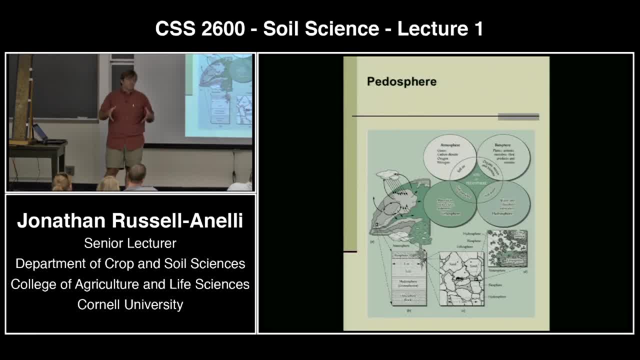 I want you to think of soil as a volume, okay, Because soil is not just made up of organisms and rocks and organic matter, or minerals and organic matter. It's also made up of water and air. And when you start thinking about water and air, you have to start thinking about a dynamic. 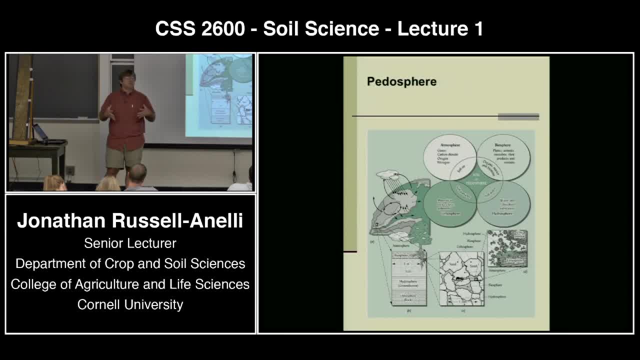 system. It rains. What happens to your soil volume? What happens to it? It rains, It fills up with water. So, if it fills up with water, what happens to the air? It what Less air. Say it again: Less air. 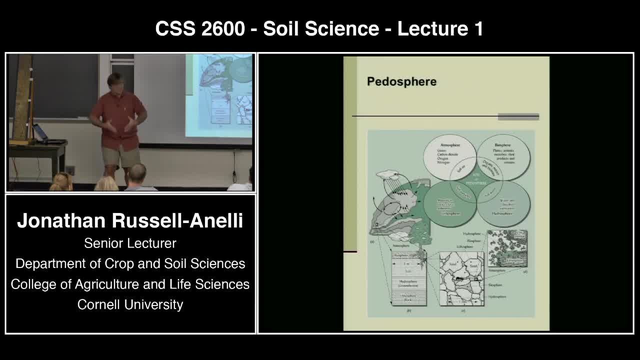 It's less air. Where does that air go, though? Well, sometimes it can be pressurized. Most of the time, when the water goes in, the air comes out, Or it goes as a front end of a leading. you know the waterfront. 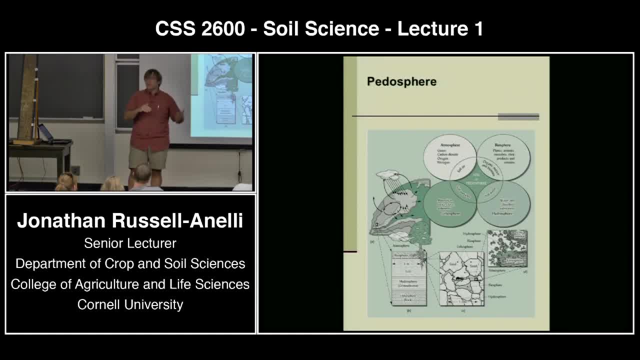 Water's pushing this way, You have forced air coming throughout. Has anybody gone into? and this is not quite the right analogy, but has anybody gone into a cave, and you feel the breeze coming out. Okay, well, why is that breeze coming out? 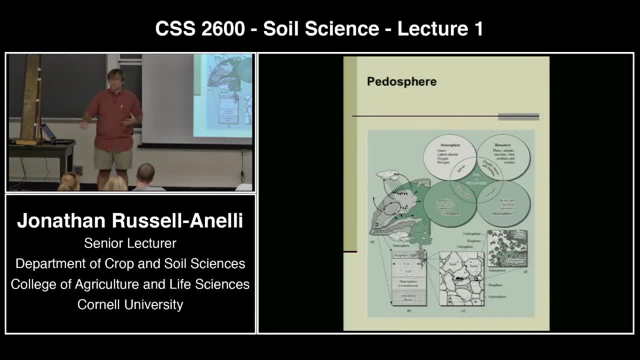 Air is rising in one location and it's creating a sort of suction or pressure. The same thing's happening with the caves that are the particles between soils. Things are pushing in, Things are going to push out. So we've got actually a pretty good handle on what soil is already. 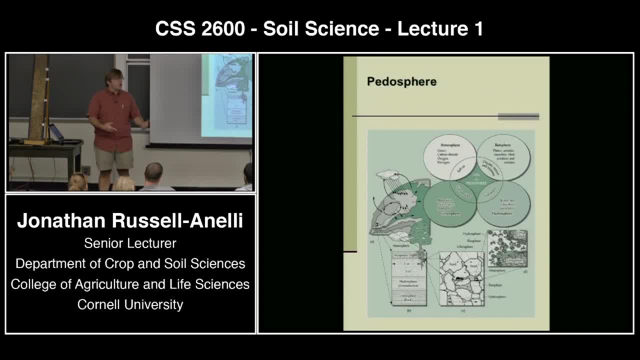 Maybe not technically, but we have an idea. It's not just the stuff that you walk on, It's not just the stuff that grass grows in. Soil is a volume, And the coolest thing about soil is that soil is at the interface of four very important 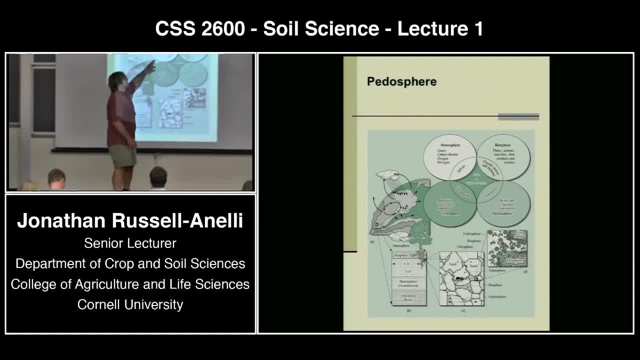 realms of the planet. The first one is the atmosphere. Okay, So I'm standing up here and this is the soil below me. There's an interface between the atmosphere and that material below me, But if soil is actually a volume of which, it's not a solid material, that atmosphere. 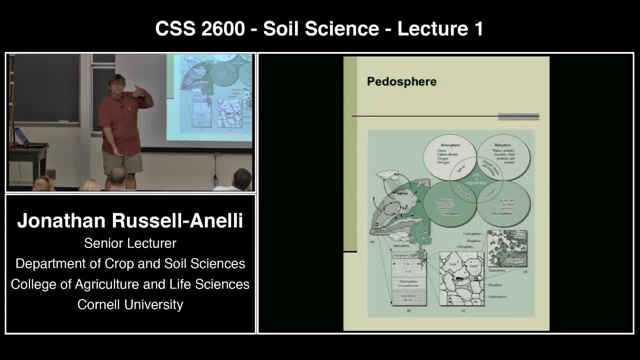 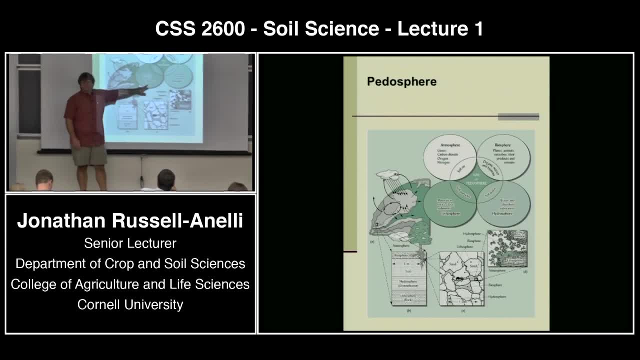 is interacting all the way down through that soil. It's not just at the surface- Okay, All right, It is also the interface between the lithosphere, the rocks- Okay, It is the interface between Up here and the bedrock down there. 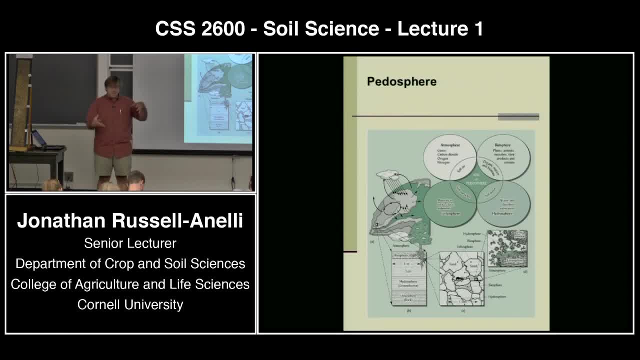 Does that make sense? Okay, Things happen at the exchange sites. The exciting part of ecology and systematics is at the edge. Has anybody ever heard the edge effect? Edge effect- Does that sound familiar? It's what's happening at the edge. 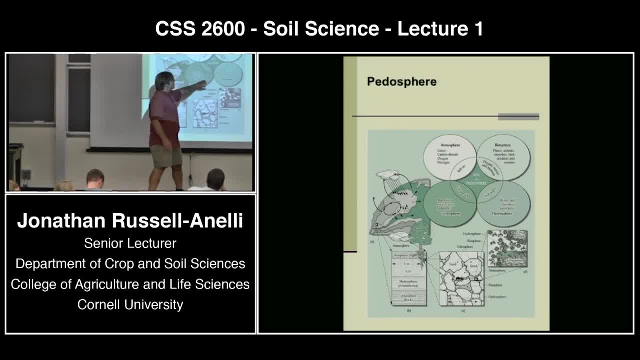 And soils is the edge. It's also the interface between the hydrosphere. We just talked about the rain. It's not just the rain, It's groundwater, It's the oceans, It's the rivers, It's that interface. 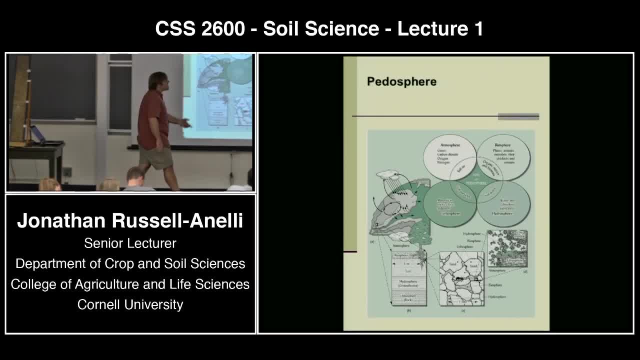 It's the dew, It's the interface between all of this and it's the interface of the biosphere. I'm sure all of you guys have sort of heard, even though this is he never actually said this, but there are millions and billions of stars in the galaxies and he never actually 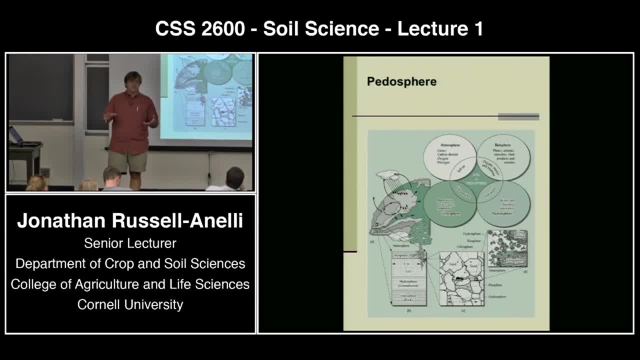 said that. Does anybody know who I'm talking about? Carl Sagan, Carl Sagan, Okay. Well, it turns out that there are, in fact, millions and millions of organisms underneath our feet. There are more organisms underneath our feet than above it. 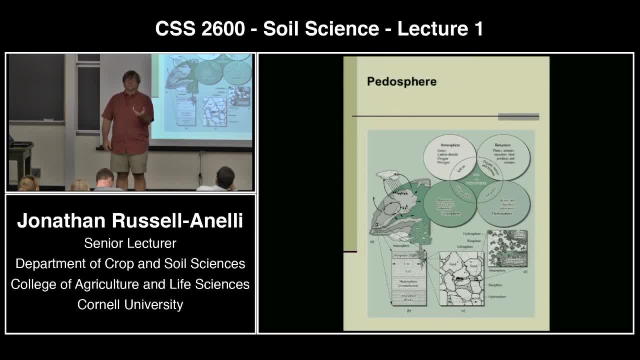 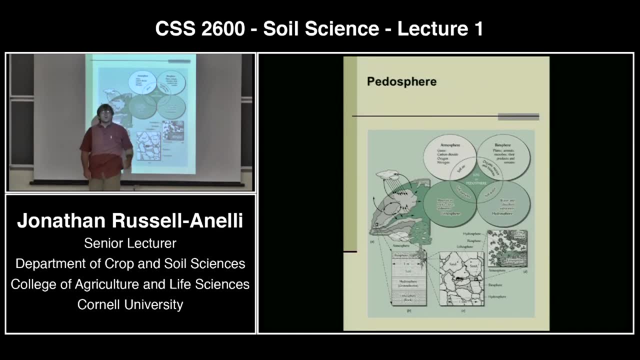 The tablespoon of soil that has a million organisms in it is legitimate, though it is somewhat selective- You've got to take a certain type of soil to do that- but it really is there. So it really is interface Soil sits in this Venn diagram between these four very important realms of our planet. 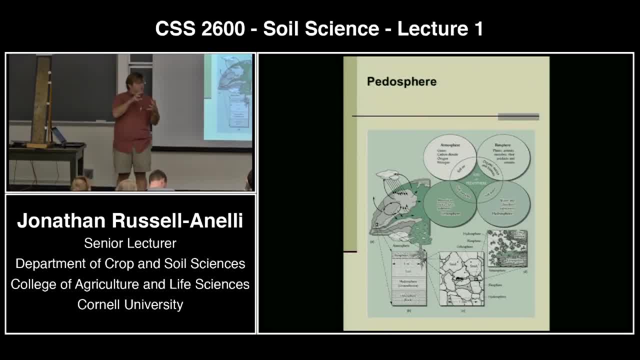 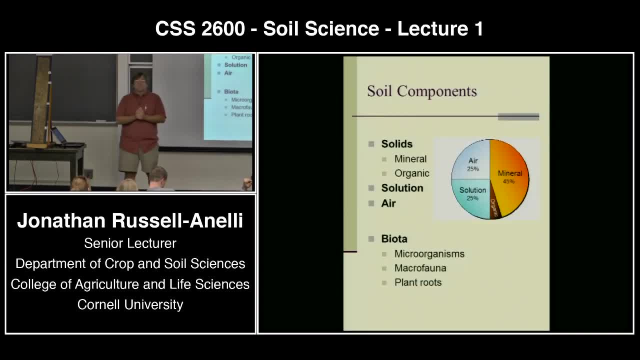 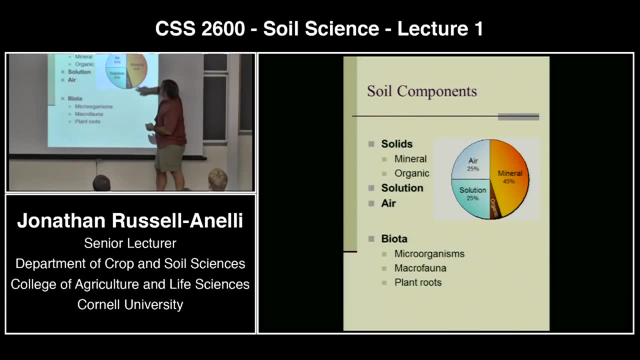 And it's a volume. It's not just a thin skin, It's a volume. Okay, So let's talk about that volume. Well, there are basically four components to that soil volume. The first, and the one that most people think of, is this mineral component. 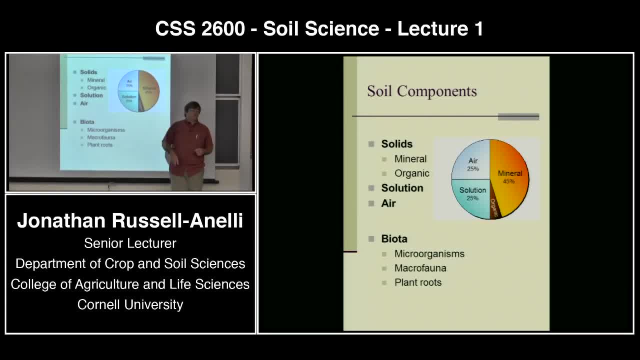 Basically 45%, and about 5% of it is organic, living and dead. So in an idealized soil this is that circle. 50% of that soil volume is actually solid material, 45% of the total is organic. 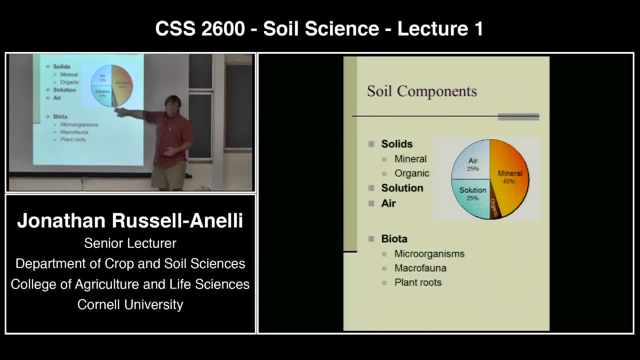 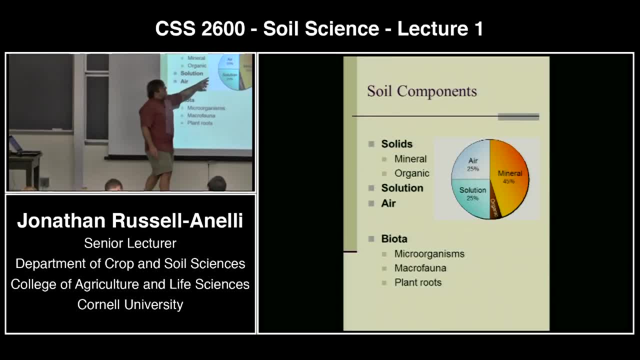 Okay, So that's the mineral. 5% is organic, The other 50% is air and solution, or you can call it water. Okay, Now, very easy to say: this is 45 and this is 5.. It basically is: 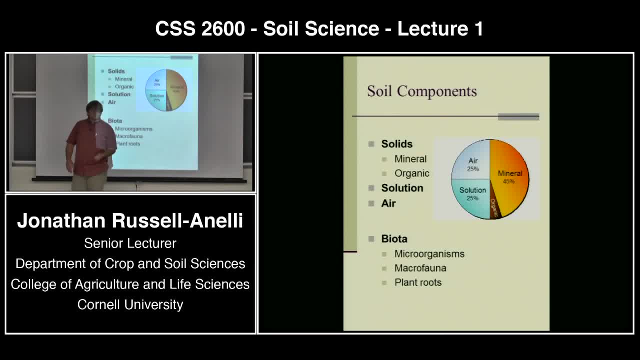 It's not so easy to do this. It's not so easy to say 25% is oil and 25% is solution, Because what happens when it rains? Well, that solution component is going to get a lot larger And we're going to lose that. We're going to lose the air. Give it a couple of days and water drains out. the plants start respiring, they start sucking up that water and all of a sudden, this solution starts getting down here. And, as we're having much part of the country right now and we had an Ithaca for a significant 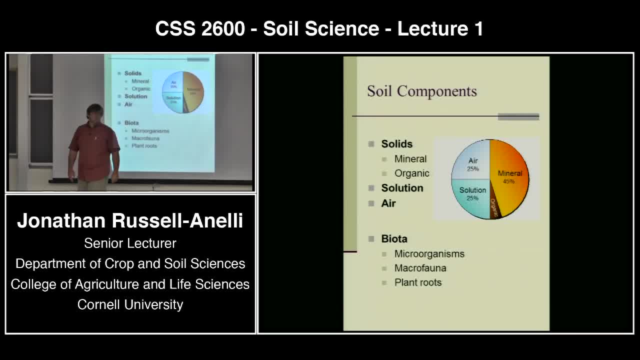 part of the summer you can get this so far down that you go into drought conditions. So this half is very dynamic, very, very dynamic. It turns out that this side is actually fairly dynamic as well. Okay, So you're going to have a lot of soil material all over the place. 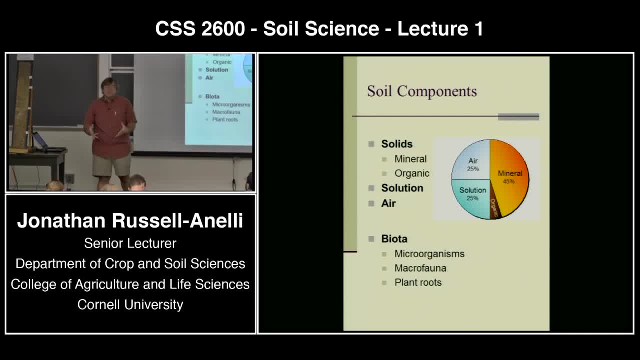 Depending upon how you're managing, depending upon what type of organisms are living in the environment that that soil is located, this organic matter can be as high as 100% or 50%, I should say to as low as zero. Can anybody think of a situation where it would be 100% or 50%? 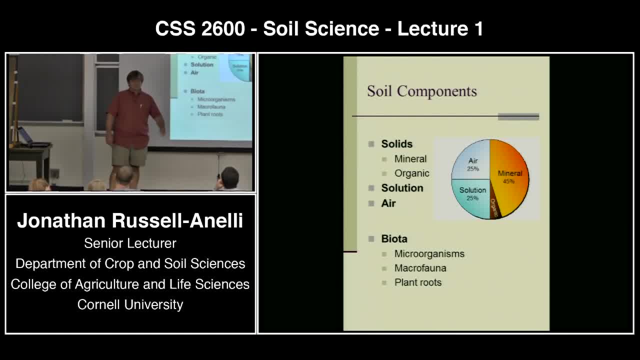 Go, Compost, Compost. Really good one Compost, Another one, Wetland, Wetland, So hydraulic wetland type of system. So we're looking at organic soils, 100% organic soils. Two Very good examples. 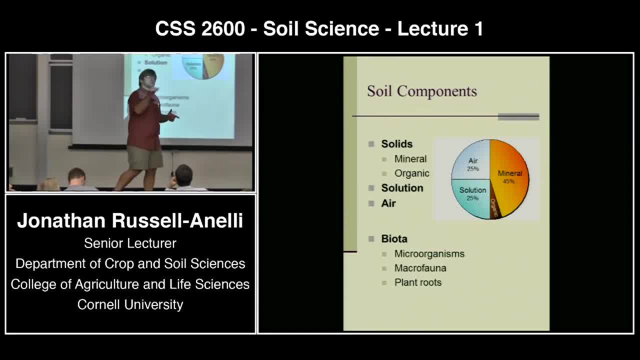 Go Tundra soils, Tundra soils. in some cases those are pseudo wetlands in a sense, because they have accumulation of organic matter. The accumulation of organic matter is not because of water, which we usually have with wetlands. The accumulation of organic matter in that case is because of cold. 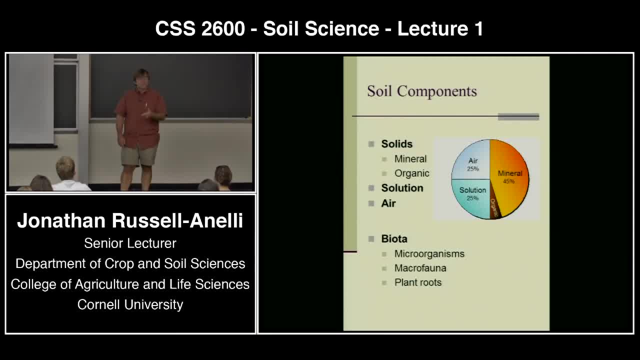 In both of the cases- water and cold- you're having accumulation of organic matter because you're having a reduction in decomposition. The system goes wet. what happens to decomposition? It stops or gets really, really slow. Why There's no oxygen. 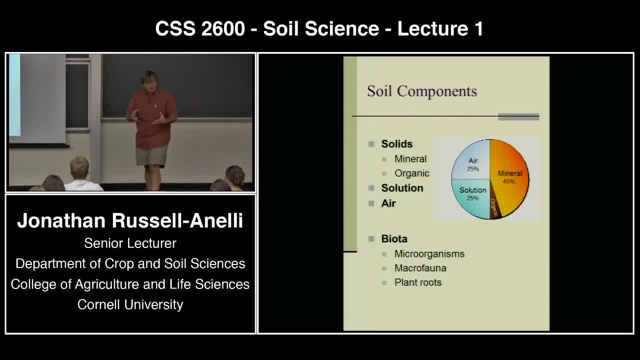 The microbial population that's doing the decomposition or the microfauna population that's doing the decomposition stops respiring. They can't respire, They can't do the decomposition. The same thing happens in the tundra: The system goes cold. What happens? 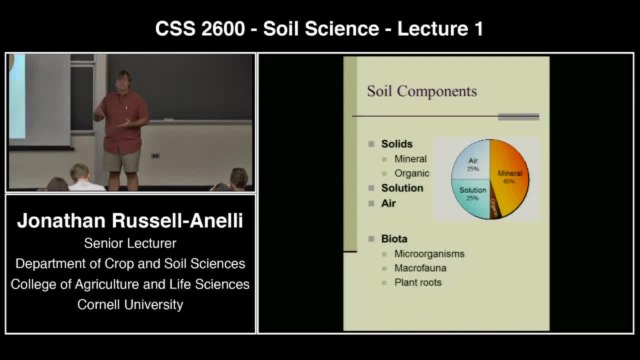 Organisms stop doing their stuff. We have accumulation of organic matter. Make sense This organic section and throughout this entire volume. we also have biota. This is the comment that we made earlier that soils are also organisms. This is microorganisms, macrofauna as well as plants. 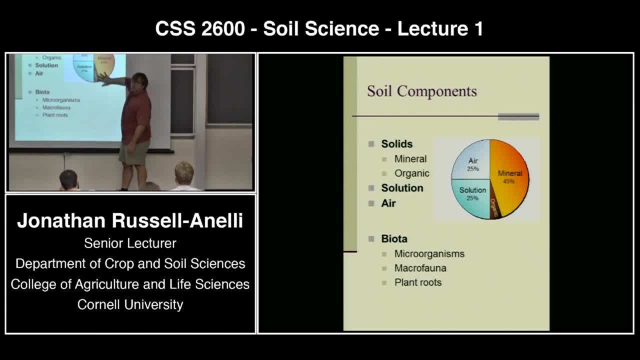 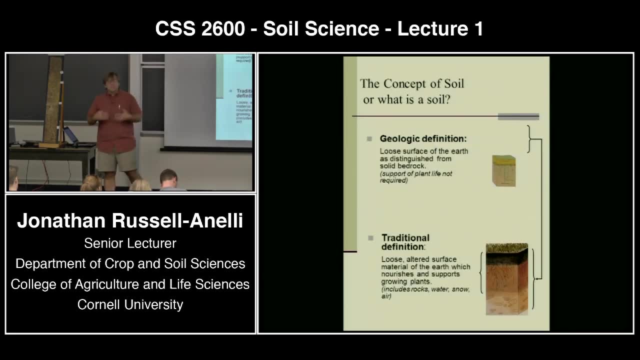 Very large community of biota, Large variation in this and huge variation dynamics in the water and air or soil solution and air Questions. so far Cool. Let's get to the technical end. I already threw this out there. What do you think of the soil? 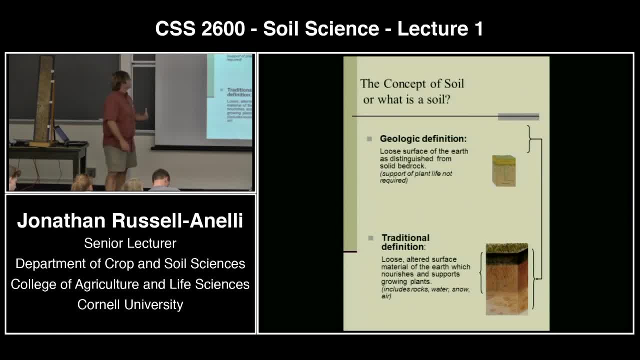 There are a couple of technical concepts, technical definitions. There's a geologic definition as well as a traditional definition. Geological definition is basically loose surface material between the boundary ground and soil. There's a geological definition as well as a sort of traditional definition. 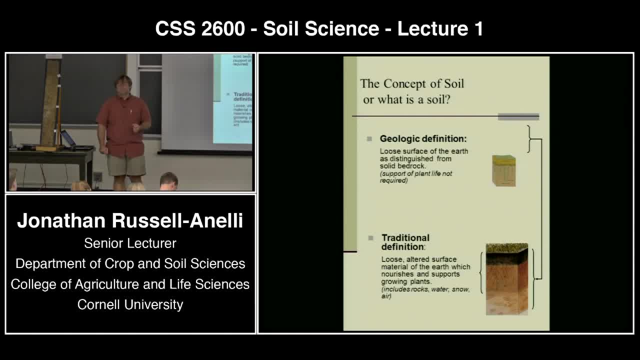 layer of here and the boundary layer of rocks. this loose material. there's no requirements on it, it's just loose material. okay, traditional is this loose altered surface material of the surf surface that in some cases- and in this case includes rocks, water, snow, air, etc. but is capable. 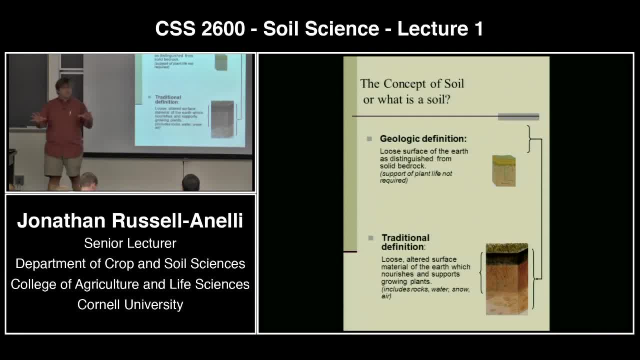 of growing plants. those are sort of the two definitions that most people operate by us being soil scientists- scientists being the operative word. we have our own real definition of what soil is, but basically it subsumes these two ideas, this loose material. material encompasses rocks, air and water and is capable of supplying nutrients and growing plants. okay, our definition. 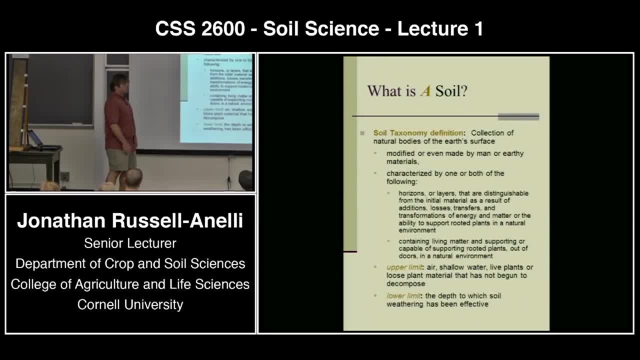 is a little bit longer, a little bit cooler. no, we're soil scientists. no, basically, it's: basically, it's saying that the soil is a material that is capable of growing plants and growing plants, and growing plants. it's saying this loose material has been modified over time. okay, the difference. 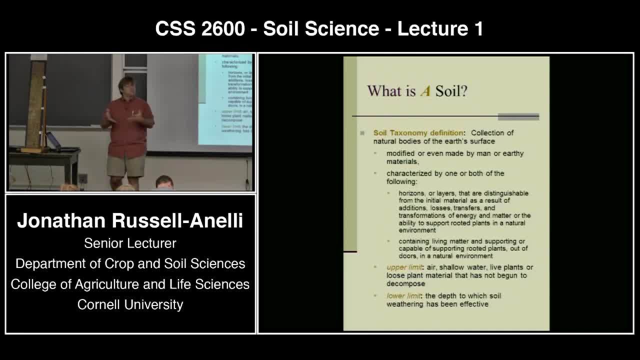 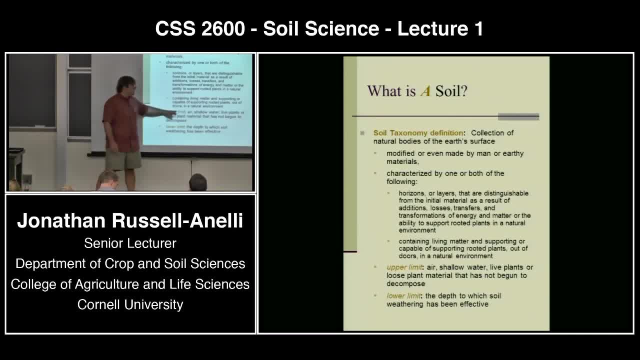 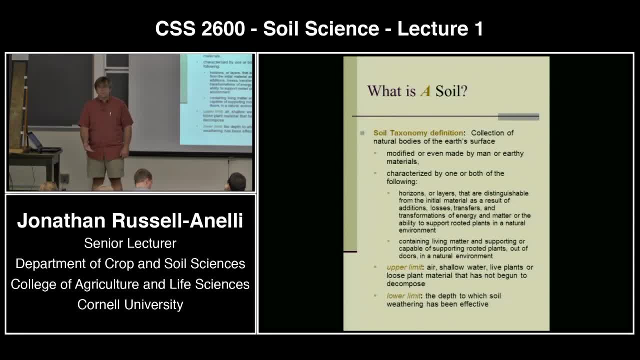 has occurred. okay, in some cases this is hard rock, in some cases this is not that far down, but it's basically sitting on top of a pile of sand or something like that. does that make sense to every everybody? But it encompasses these two traditional views that most people sort of think of as 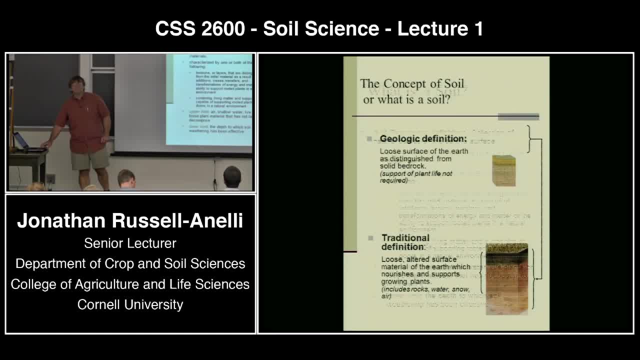 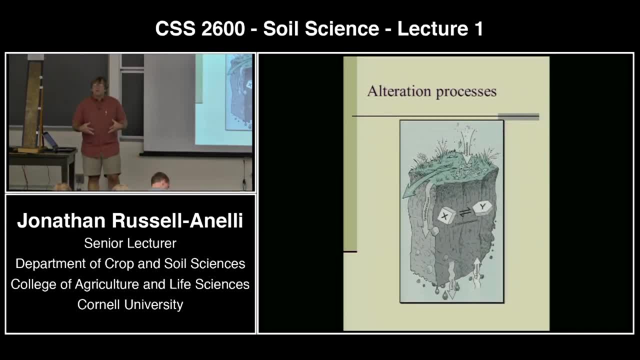 soil. Okay, questions so far. So I have sort of introduced this idea a couple times. but soil versus dirt soil undergoes some sort of alteration that produces soil. So let me introduce those alteration processes. What are they Now, you guys, I think without even looking. 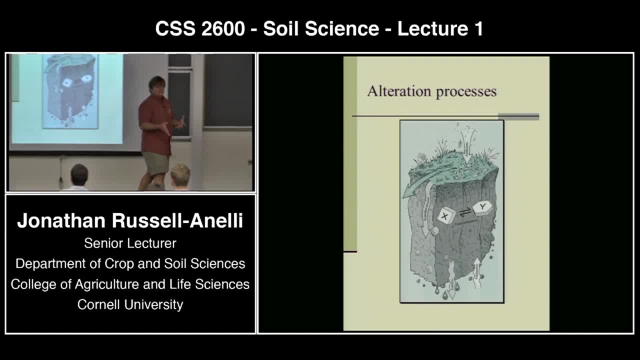 at this. without even looking at this, I think you guys could come up with all of these. Okay, what are the things that you think that happen in the real world that could potentially alter some material in it? First one is: things can be added to it. right, You got a landslide. 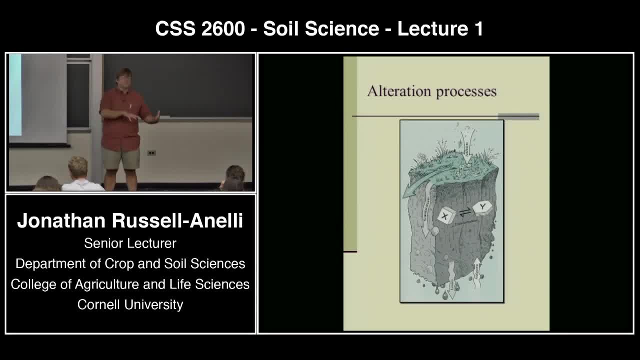 you have a wind event, you have a flood, stuff comes in, dust comes in from the air, things get brought in by water. Okay, that is an alteration process. I have material here and something comes in and alters it by adding. Okay, those same processes could also remove, So we also could have additions, but we 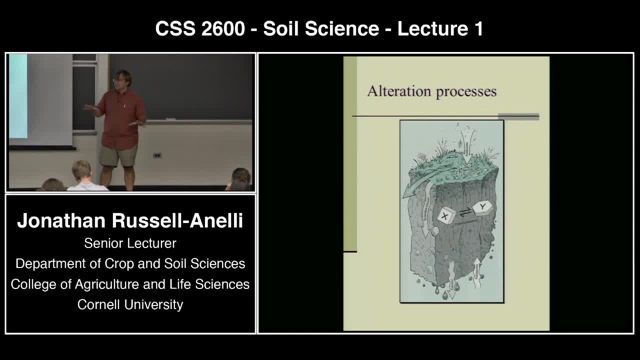 also could have losses. Does that make sense? Now, the one thing to think about when you talk about additions and losses. most people, when we think of additions and losses, we're talking about the surfaces. Okay, a windstorm deposits stuff right on top, But the truth is you can have additions. 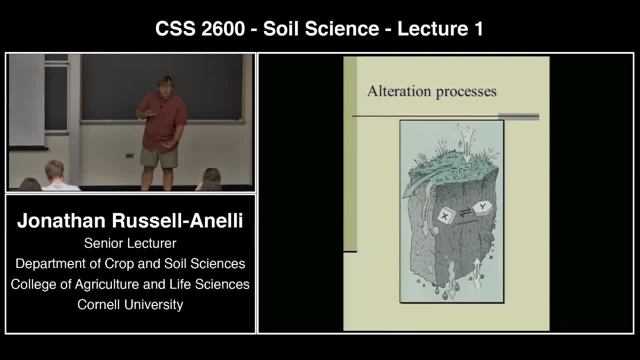 and losses coming in and out of the soil. So you can have additions and losses coming in and out of the soil. So you can have additions and losses coming in from below because you have water coming in from below. If the water has something entrained in it or dissolved in it, that material can be. 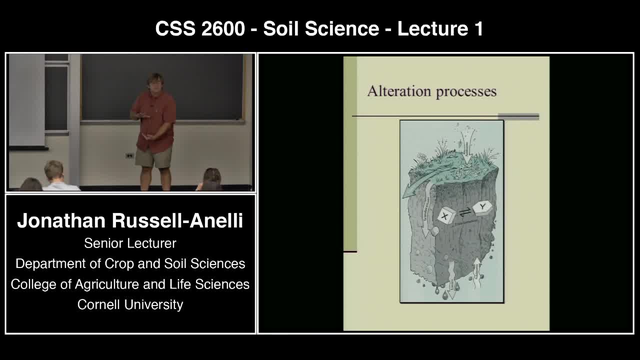 put into the soil. Does that make sense? It also can leach stuff away. If the water comes through a material and leaves that material as groundwater, it's going to potentially dissolve materials that are in that media and take it away. Okay, so it's not just on the top, it's throughout that whole. 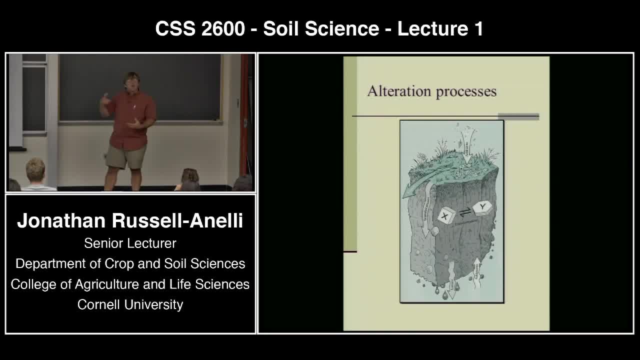 volume of material. Okay, now if I have water moving into the system or I have heat transfer- I mean sunlight comes down- I can also have alterations. The material doesn't move, but it changes in space. Okay, I'm sure most of you guys are taking chemistry. Okay, if you put a solution in with another thing. 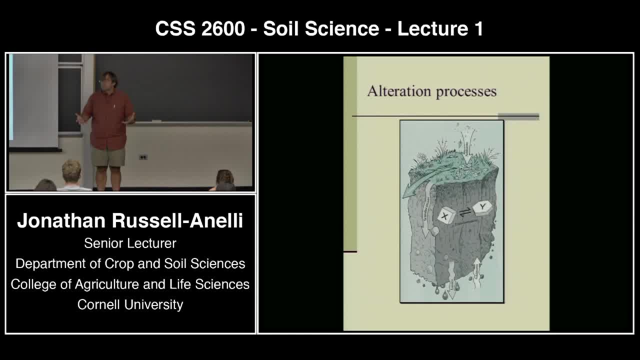 you mix it up, you can potentially make something else, right? Has anybody made rock candy? Look real simple. okay, You put sugar into boiling water and you put a string in it and you basically let it cool and let the sugar crystallize. 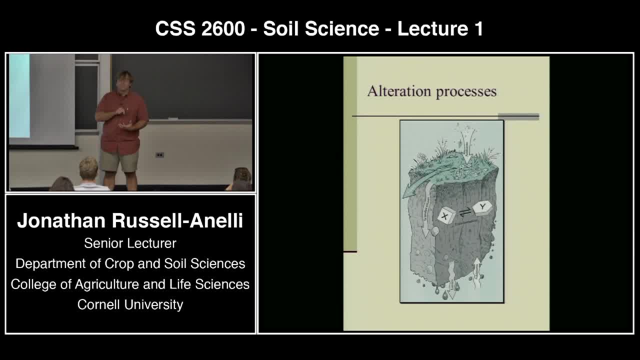 It's still sugar, but it has altered its form. That kind of stuff happens. That's an alteration. That kind of stuff happens in soils. We have crystals forming all the time. They may not be sugar, so I'm not suggesting that you go out there and eat dirt, but it's. 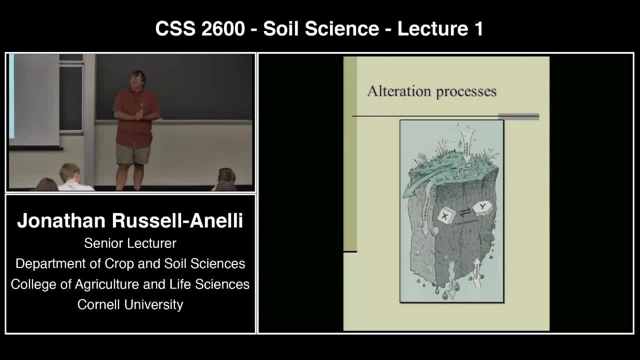 an alteration, It's cool. Last one is a translocation. Translocation just means move. You can certainly imagine if it rains up here, that water potentially can entrain something or carry something in it and move it down into the soil and move it to a new location. 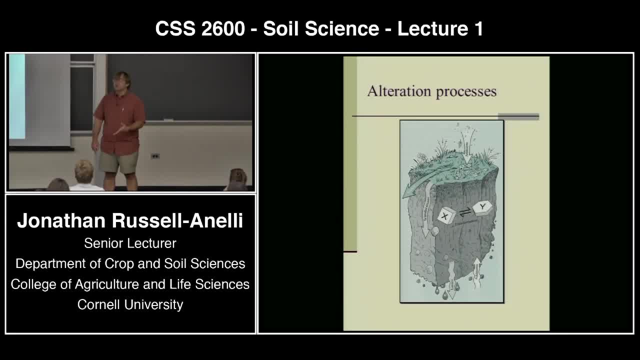 In fact, next week, the first soil that you guys are going to see is a classic example of this entrainment. Water rains, Water rains. Rainwater hits the ground, Entrains or puts into the water Water column Very small clay particles. 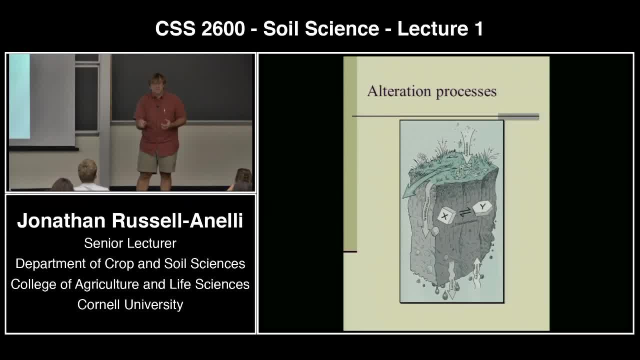 Those clay particles move through sand and get deposited farther down. That's a translocation. Does that make sense? Okay, Go. How is that different from things being added That is within the same volume? If I have clay, that's at the top and it's being moved down into the same volume versus. 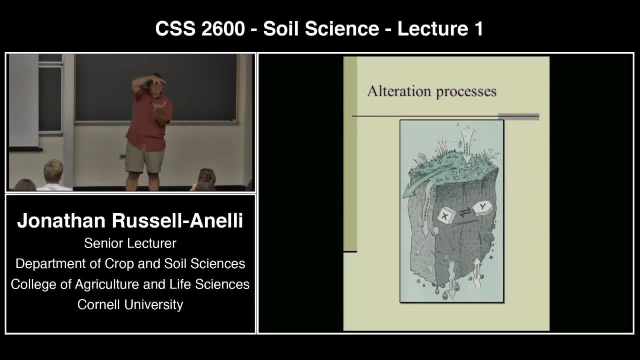 clay coming in or nutrients coming in from water into that same volume. That's a translocation. That's a translocation. Now that actually brings up an interesting question: What is your definition of the boundary? My volume is here, but if it's a little bit larger, the water actually may be coming from. 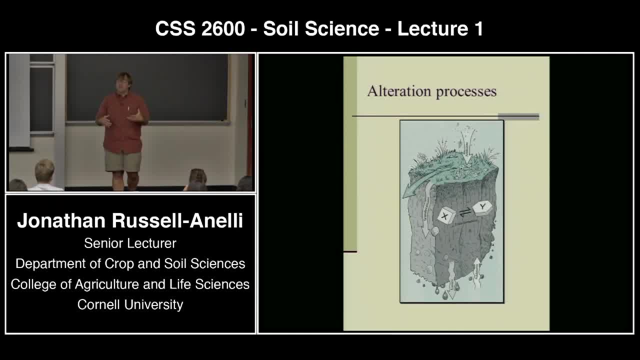 the same condition. We will actually talk about that, because part of this course is about how these soils vary across the landscape, how the landscape modifies that soil. That is a very appropriate question for that. Okay, One other thing: We're still on translocation. 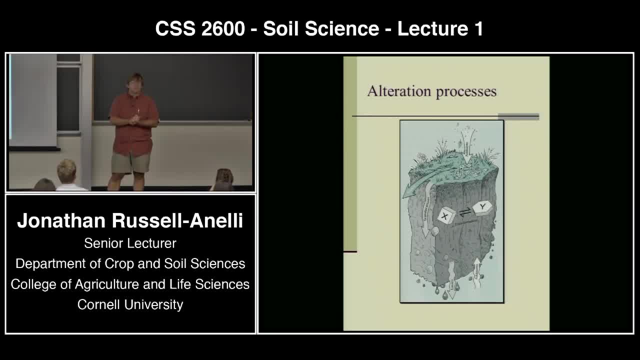 Has anybody walked through the tunnel between plant science and man library? We do it all the time We go into mandibles or something like that. Has anybody ever- Now this is the part that may be tough- Has anybody ever actually looked at the walls? 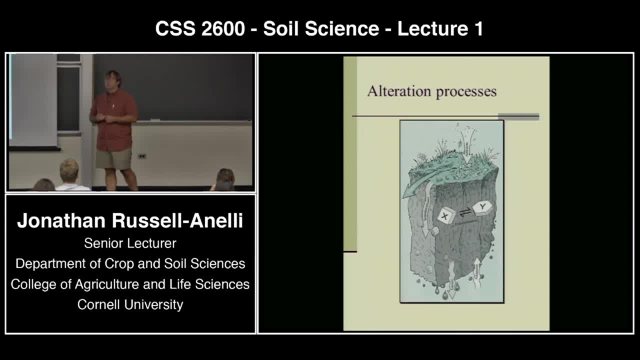 Has anybody ever noticed that there are salt stains on those walls? If you haven't, go in there and take a look, Walk down that hallway, And it's If you're on the left and a little bit on the right if you're coming from this direction. 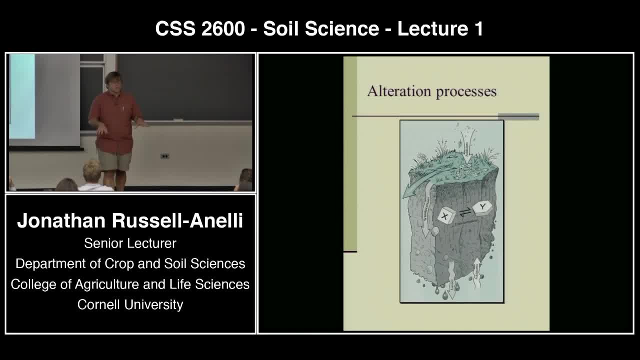 there's salt stains on the walls And basically what that is coming from is coming from wicking Water is coming in, moving down. I mean it rains, it snows. you guys have been in Ithaca a while, you know what happens, okay. 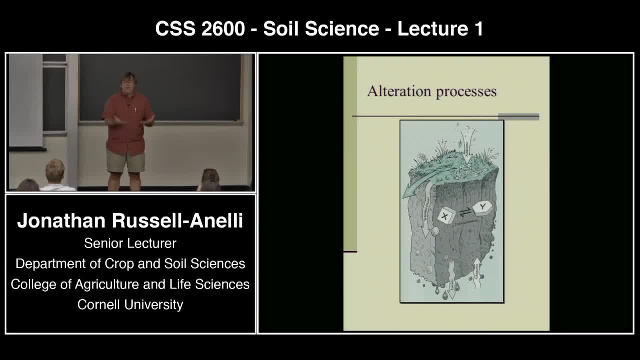 Water hits the ground, it moves along surface and then it hits the surface walls and basically starts moving up. okay, Capillary action, wicking right. You guys saw this happen when you were kids with straws. Okay, You put a straw in water. what happens when you pull it out? 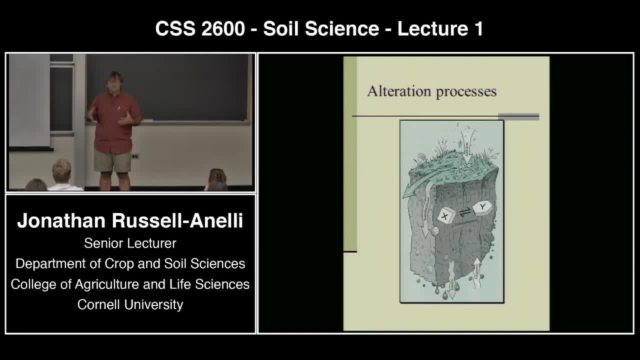 There's a little drop of water in the end, right, Okay. Well, what's happening is that water is entraining dissolving salts. There's a lot of salt around here Every time it snows. what does Cornell do to the sidewalks? 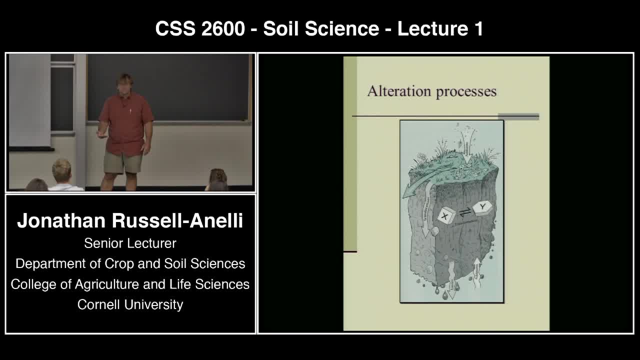 Covers it with salt right. Well, the water that comes in there, that dissolves, solubilizes that salt, puts it in the water. That water then runs in down the tunnel, hits those walls and starts climbing the. 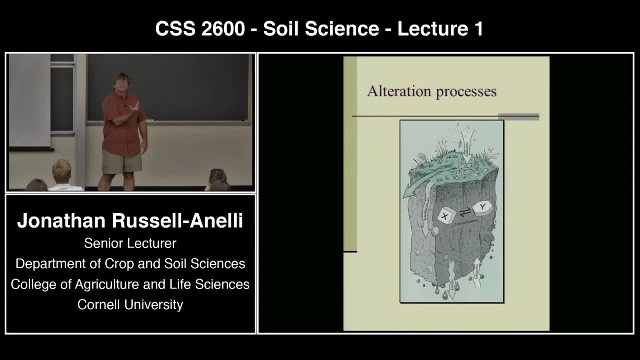 walls. That's the capillary action. Well, sooner or later, that water is going to evaporate. and what's left behind? The salt? Well, the same thing happens in soils Around. here it's not a big deal, but what happens if you're out in the west or in the deserts. One good rainstorm solubilizes all the salts. water moves into the soil but doesn't make it all the way down, actually starts coming back up because of evapotranspiration. It goes down. It solubilizes all the salts. 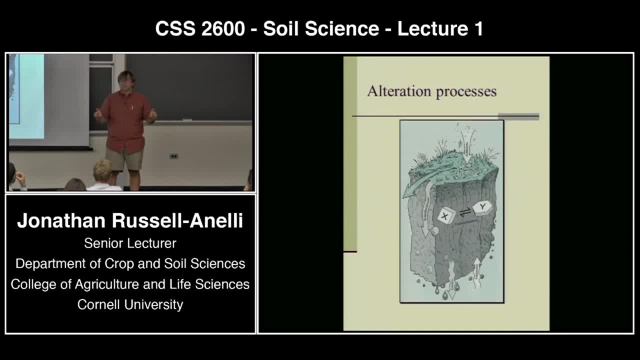 Comes back up, evaporates and leaves the salts behind. Does that make sense? I will be showing you some pictures of this later in the semester. This is one of the really cool things about this translocation. Translocation doesn't just necessarily go down, but it also potentially goes up. 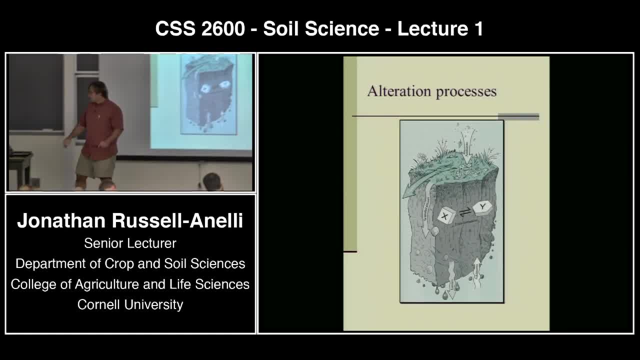 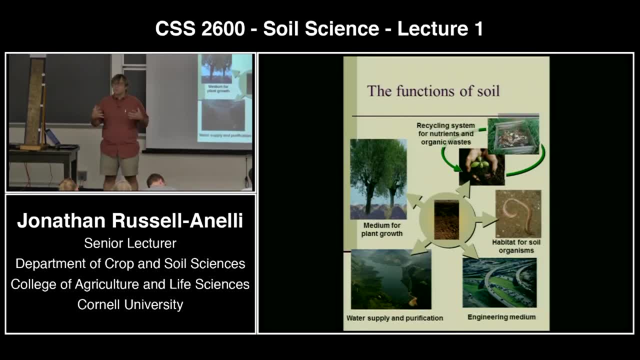 Okay, Cool Questions, All right. so we've got this volume. We have somewhat of an understanding of how this volume of material is modified and changed into soil. What the heck does it do? These are sort of the functions of that volume of material. 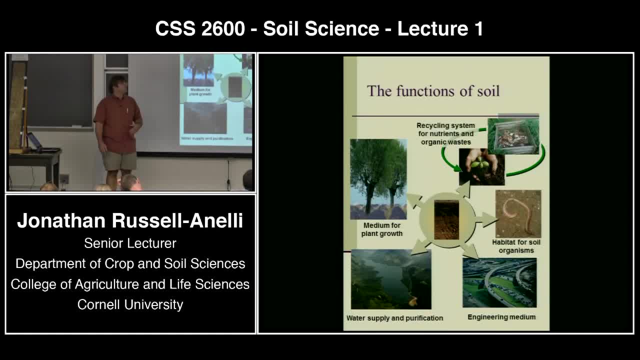 Most of these functions you guys would pop off the top of your heads. Obviously, it's an engineering medium. We build things in it all the time. We build road beds, We build buildings, We put septic systems in there. 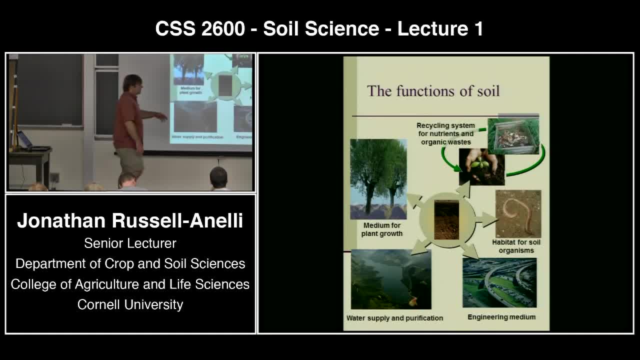 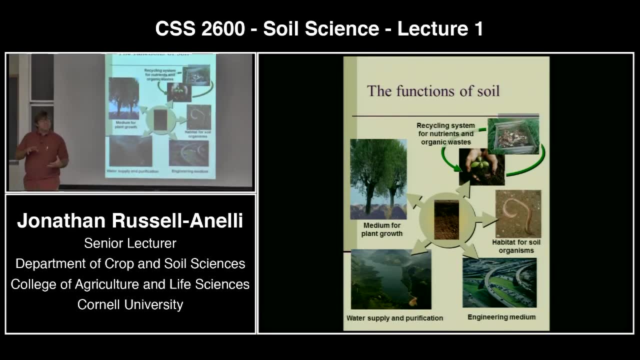 We do all different kinds of stuff, But it's not just a building material for us, human-made materials, It's also a building material for plants. Plants actually need the soil for a lot of reasons, but plants actually need the soil from an engineering sense because it needs something to structurally anchor itself. so 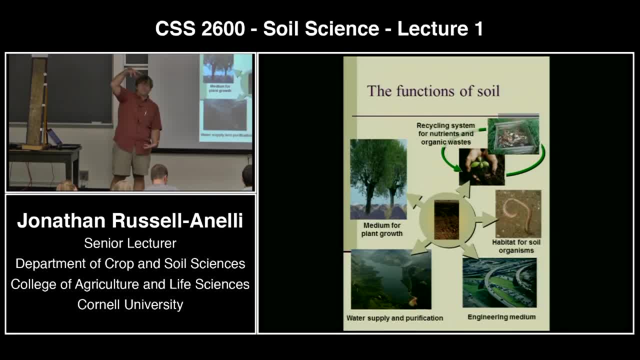 that its biomass can grow above and below the ground. Okay, There are things in the world called air plants. They don't need the soil, but most plants need that material to grow in From an engineering sense. They also need that material to grow in from a growth media. 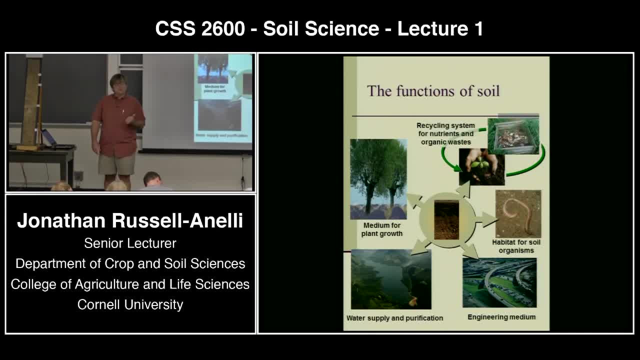 The soil is the major supplier for most, if not, with one exception, all, of the nutrients. It is the way we get it: We get it, The plants get it, which ultimately we get. Okay, So this media is the nutrient supplier and it's also the water supplier for plants, and 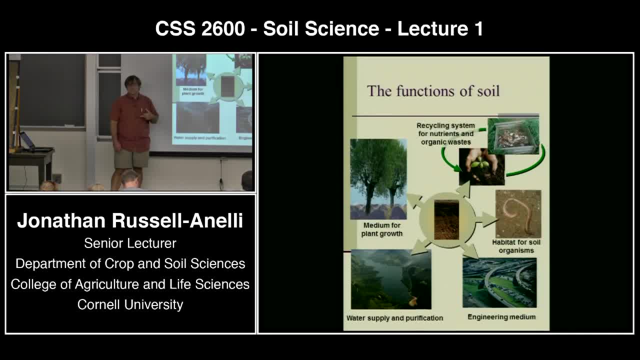 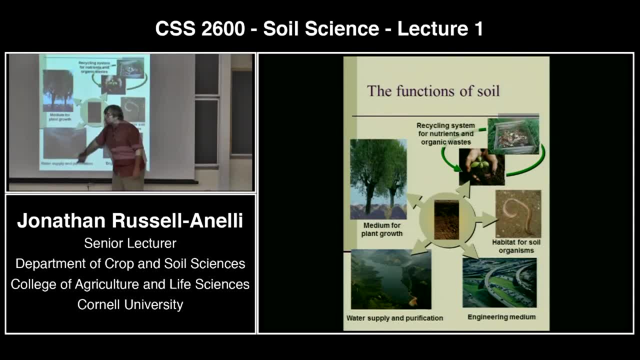 for us And, ultimately, the plants for us. Okay, It also. so it's recycling this nutrients, putting it into here, It's getting the water, It's putting it into the plants, It's the engineering material for the plants and for everything else. 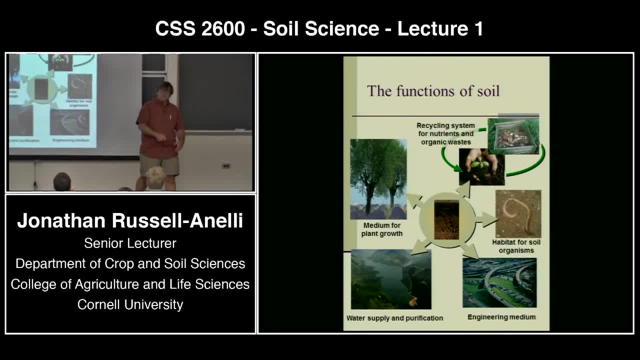 But it's also a huge habitat for these organisms. Remember me saying: there's that teaspoon of soil. How many organisms are in it? Okay, These organisms are driving much of this and this which then provides for this. Okay, They are doing the decompression. 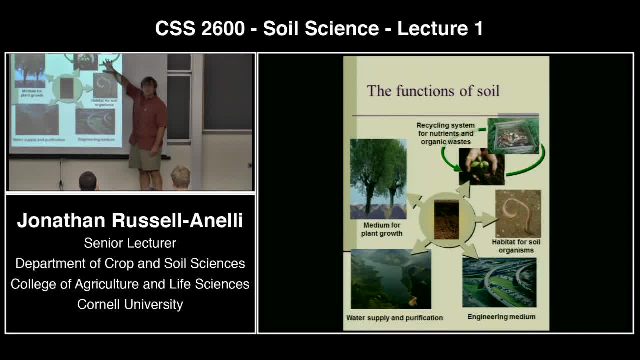 That decomposition is putting organic matter into the soil, but it's also releasing the nutrients that are in that organic matter for the plants to take up. They're also degrading all different types of organic materials which purify the water supply so that when the water comes out, for the plants and for us, it's cleaner. 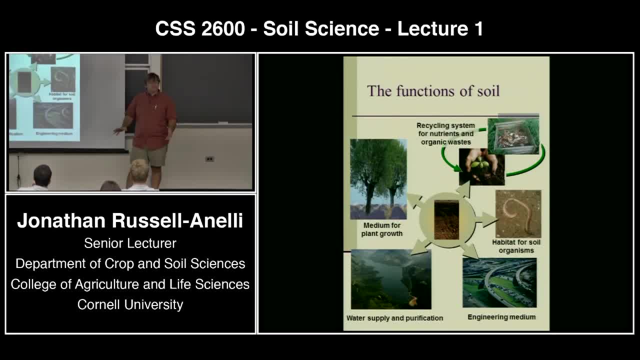 Cleaner Make sense. Yeah, So I'm sure you guys can come up with lots of examples for these sort of five functions. Can you think of some of them, Don't? you don't have to yell it out at this point, but think about it. 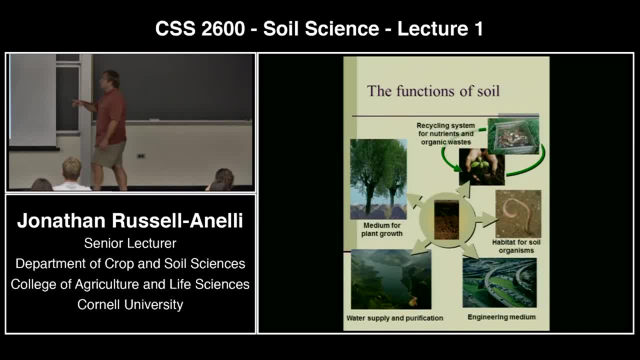 The reason I ask you to do that is because this is how we figure out the interpretations, This is how we figure out the uses of these soils. Why do we want to know these properties? Because of these five Very important functions, And if we can figure out the properties that drive these things, we can figure out different. 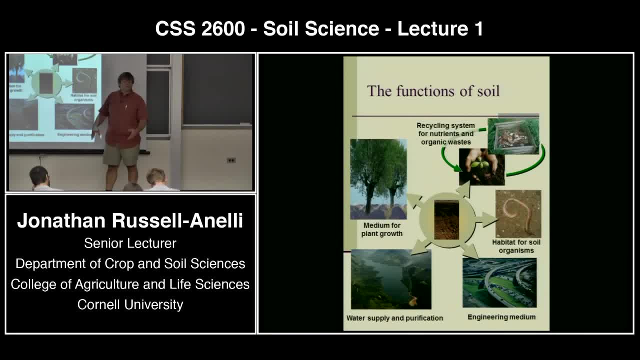 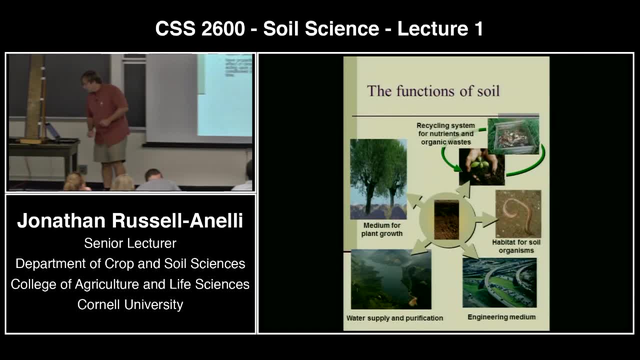 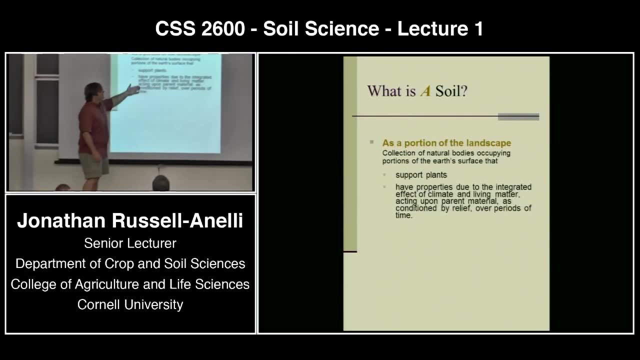 ways to make interpretations and manage the soils, for whatever goal it might be. Does that make sense? Yeah, Kind of-ish Cool. All right, Back to what is a soil. It's a portion of the landscape, supports soils and has properties that are due to. 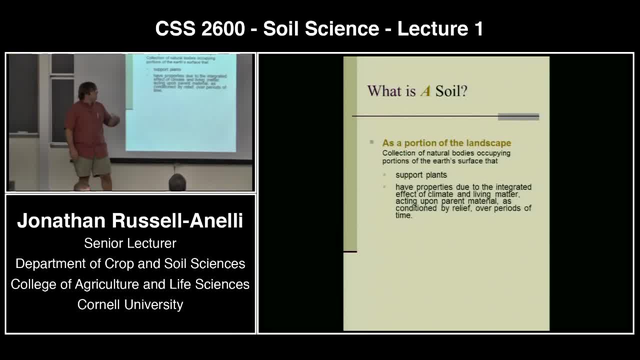 alteration but are integrated. That's the climate of living material acting upon some sort of parent material that's conditioned by relief over periods of time. Gobbligook right, This is basically the soil function equation. You guys ready for this? 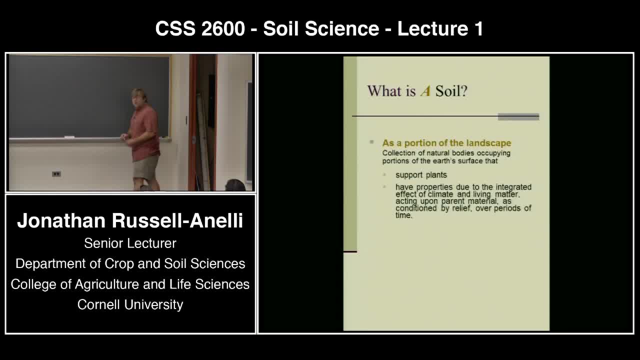 Soils are a function of five things. We call these functions factors. Soils equal a function of parent material. Okay, What is parent material? Rocks and organic material, One of our definitions of what soil is right. Rocks and organic material. 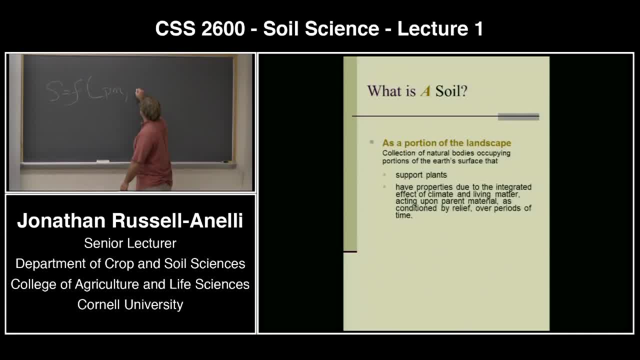 This parent material is affected by climate. What's climate? Temperature and moisture. Temperature and moisture: We've talked about both of those. As the temperature rises, biological activity increases. We talked about the tundra. Okay, As moisture rises, Potentially it increases organic activity until it gets to a point at which there's 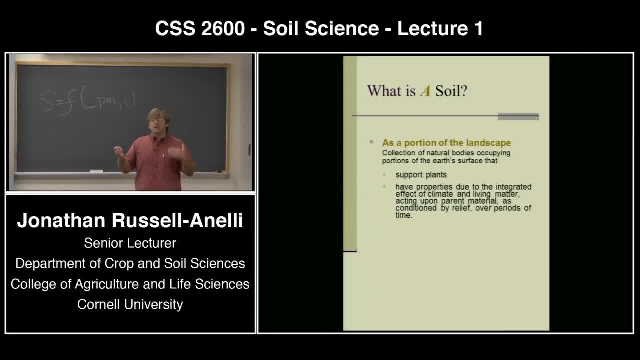 too much water and aerobic organisms basically cease operations. Now that doesn't mean that it's not anaerobic organisms and it doesn't mean there's not organisms out there that have figured out how to function in water. But if there's no oxygen in the water, not like fish can figure out how to swim in water. 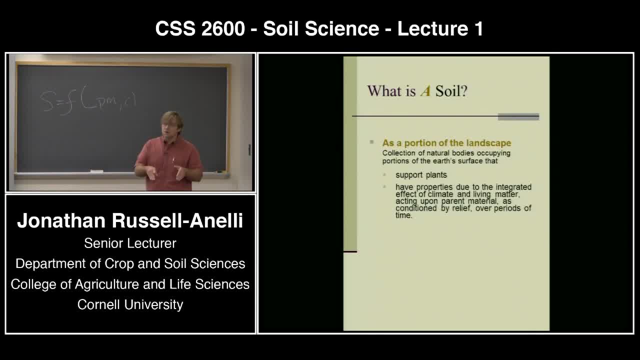 but if there's no oxygen in that water, the fish can't survive in the water. Okay, Does this sound familiar? Eutrophication and things like that. So climate drives a lot of the biota. The next one is biota. 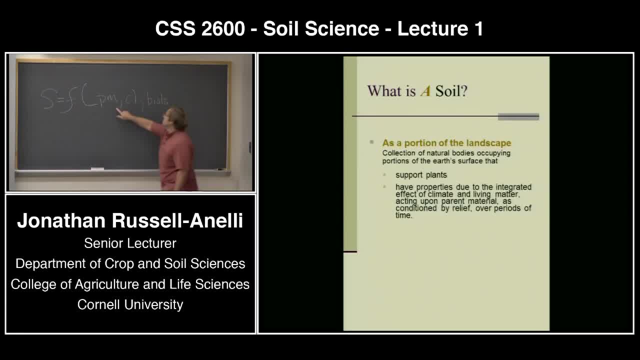 The organisms. So one, two, three. The distribution of biota and climate and parent material is also affected by there. we call it relief, but I'll call it topography. Okay, The shape of the land. Okay, If I have a flat surface versus a V surface, what's going to happen to the water? 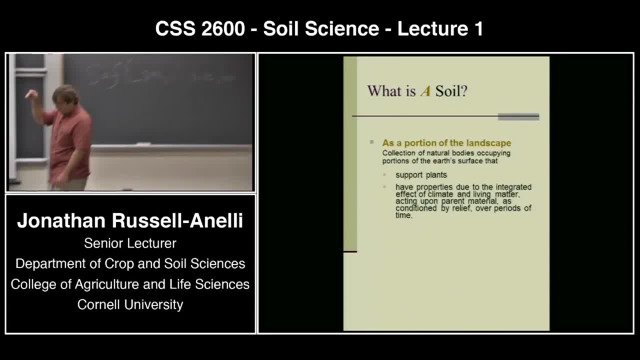 It rains and I've got a nice flat landscape. Every drop of rain that hits here is basically going to go here, And every drop of rain that hits here is probably going to go over here, And everything that's over here is going to hit over here. it's going to go here. 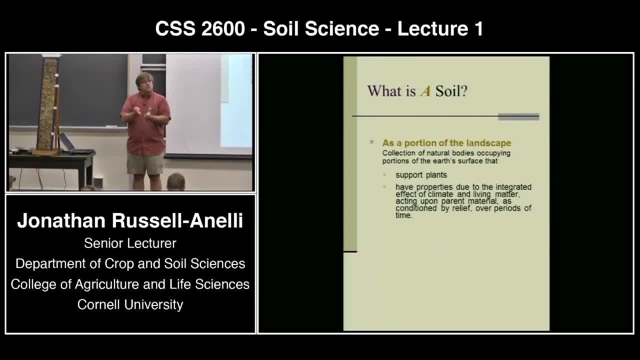 But what happens if I have a valley? It rains on the ridge. Where does the water go? It goes down into the valley. So relief is going to affect climate, Why? Well, climate's bringing the rainfall in, but relief is redirecting that rainfall to. 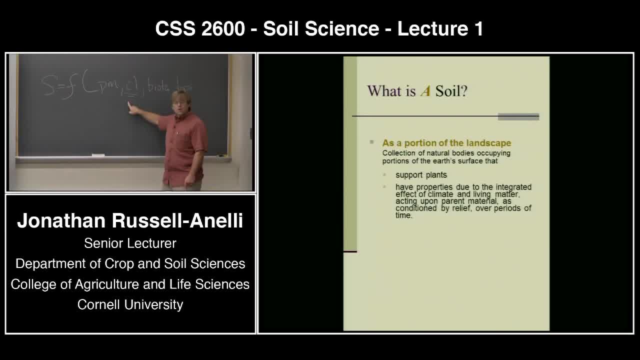 certain points of the landscape, And if I have some points of landscape that are wetter than others, I'm going to have different functioning, different soils forming. Does that make sense? And then last is time. Okay, Why time Around? here we're basically looking at 10,000, 12,000 years of soil formation. 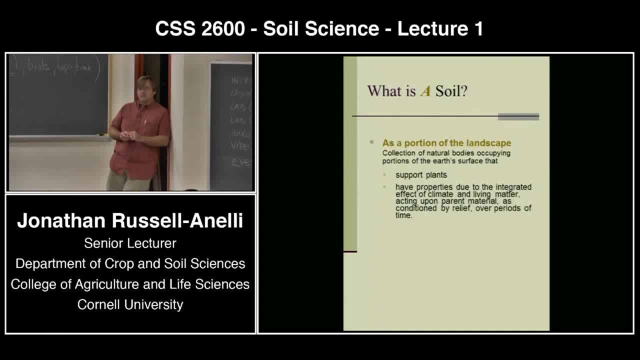 Any idea why? Glaciers, Glaciers- That's actually what the story's going to be about this afternoon, or this, not this later in this lecture, hopefully, if I don't run out of time. Okay, Glaciers. 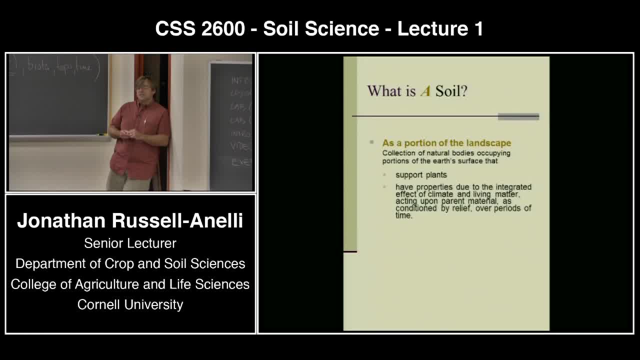 Not all the entire world had glaciers. though I'm going to say this, I'm going to say this, and you're going to hear me say this a lot of time: a lot, a lot, a lot. Okay, If you give me a weak acid and give me a million years, I'll dissolve anything. 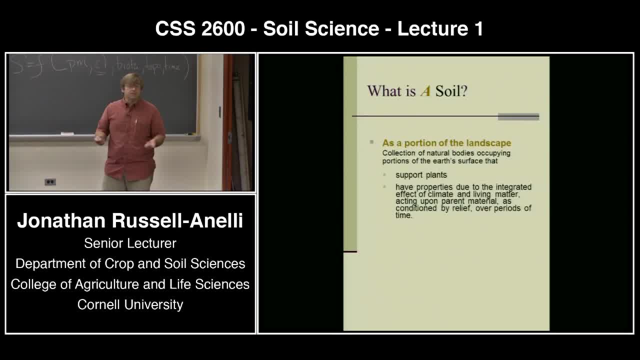 Now, if you give me a weak acid in one day, not a lot is going to happen to that material, But if you give me a million years, I can basically dissolve anything. Does that make sense? So if we're talking about a material being altered to form something, time has a huge 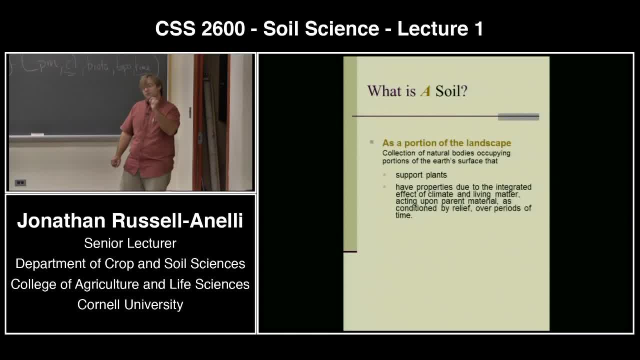 impact. Small cumulative incremental steps over a million years is going to totally change a material. Small incremental steps over a week isn't going to change a lot. Does that make sense? But that's also dependent upon the material that I'm acting on. 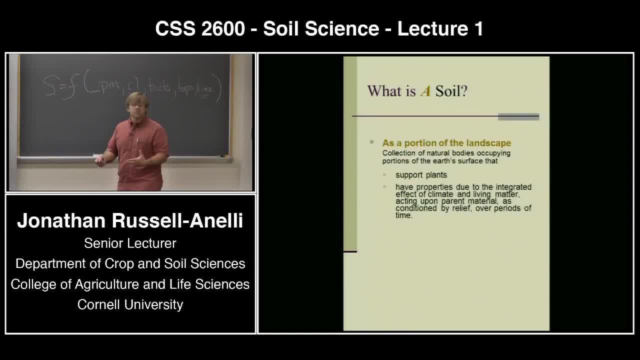 If I'm acting on a really resistant material, it's going to take a million years. But on the other hand, if it's a material that I can basically break up in my hands, it's going to take a million years. But on the other hand, if I'm acting on a really resistant material, it's going to take. 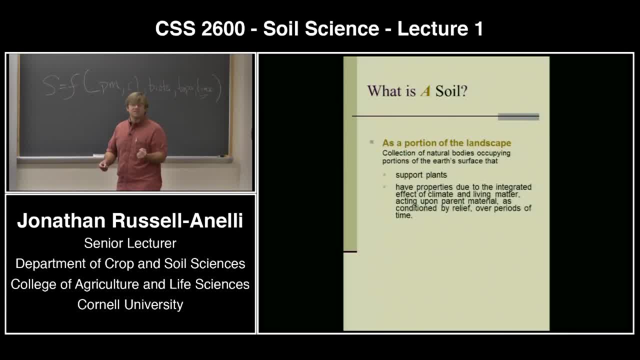 a million years. But on the other hand, if it's a material that I can basically break up in my hand, it may just take a week. Does that make sense? So that takes us all the way back to the nature of that parent material. 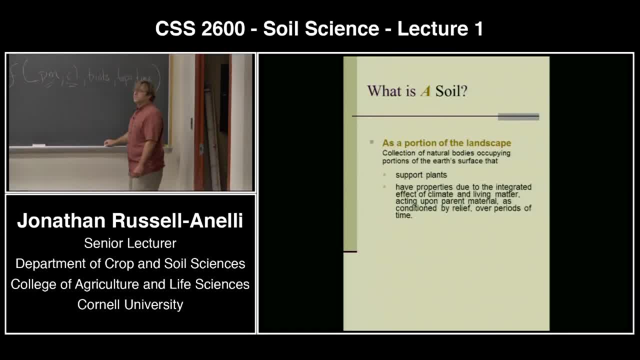 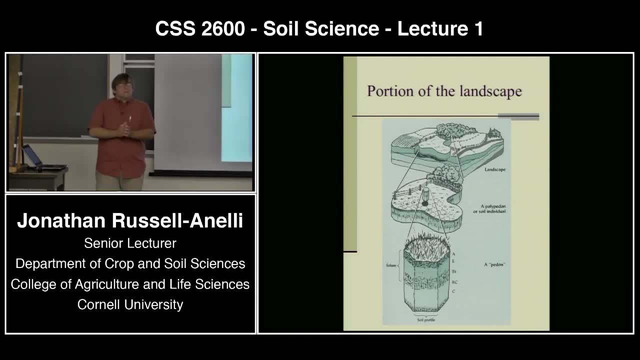 So all of these are interacted or interrelated. Does that make sense? everybody, Which brings us back to this component. Does that make sense? now, Big, long gobbledygook. Now next part of this. Okay, So we've been talking about soils as if it's just like one spot, very discreet. 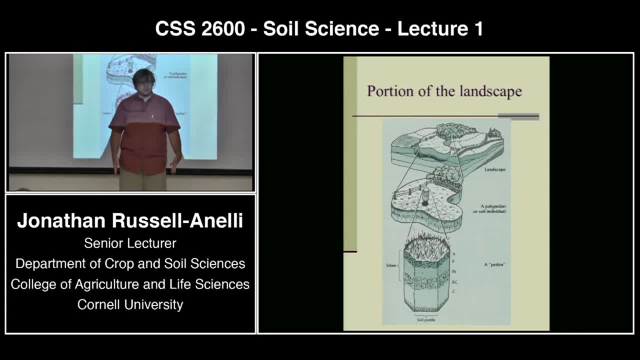 It's right here, And then there's another one that's over here, because there was the ridge and here's the valley bottom. But soils are also a very complicated landscape. They are a portion of the landscape. They're very intimately related. Here is me standing on top of a soil. 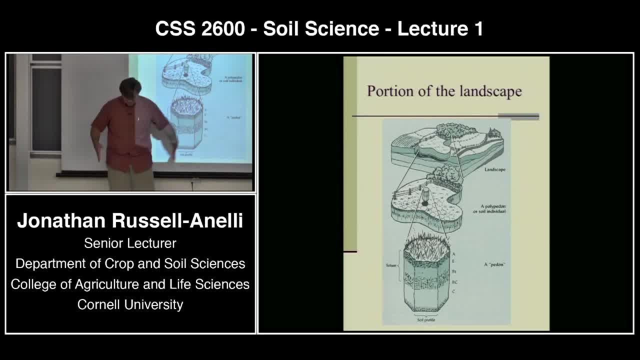 This is what we call a polypedon or a pedon. This is the pedon, This is the body that represents a soil. Okay, But if I take a couple steps over here, the soil might actually be the same material, that's. 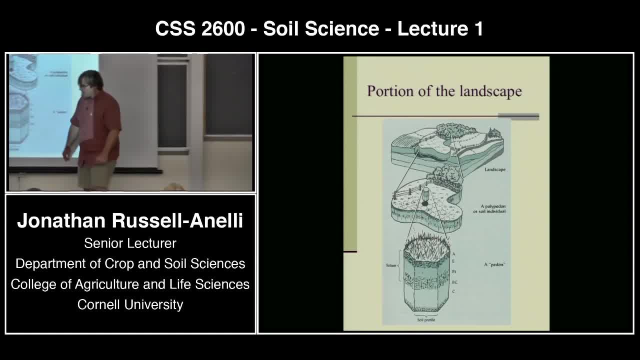 right there. Okay, So I could actually put this soil or say this pedon and this pedon over here and say, well, it's the same soil. Okay, So I can take these pedons, these individual units that we measure, put them together and 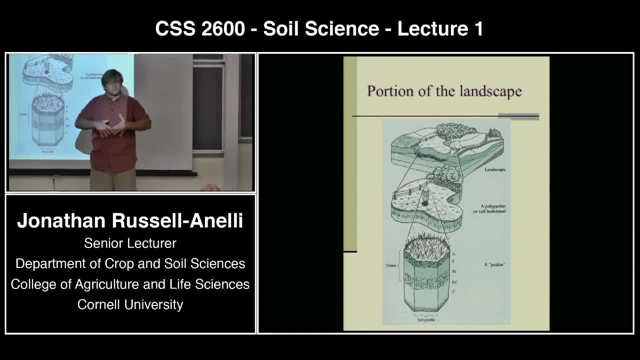 I call it a polypedon And that's my unit of soil. But if I kept walking over here and I stood on this pedon over here, it actually could be different than that soil over there. Okay. So the question then is: okay, where in here am I seeing the break from this soil to that? 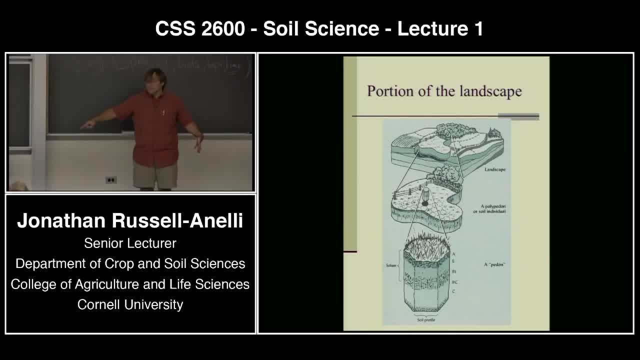 soil And, what more importantly, what is it that's making that soil different than this soil? So these soils, I mean- here's the equation, Here's that equation- Any one of these things, or multitude of them, could be the reason that this soil is different. 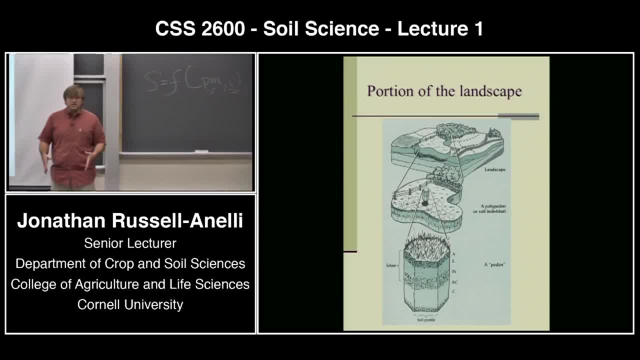 than this soil, Okay, And you will literally see, in some cases in this landscape, very discreet lines. where I step from this spot and I go over here, I've got differently different soils. But you will also see a long, a very, you know, an attenuated, not discreet at all. 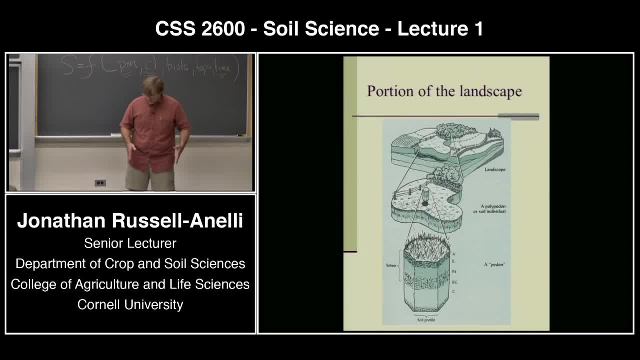 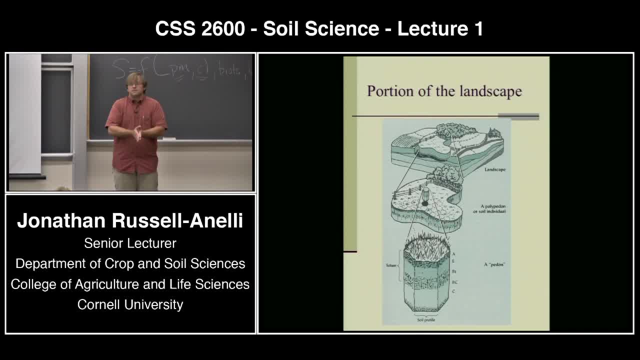 In some cases it's very discreet, In some cases it's very gradual. Okay, Does that make sense? Okay, And that's what this landscape is. We have this, the pedon which makes up this polypedon, which is basically all these little. 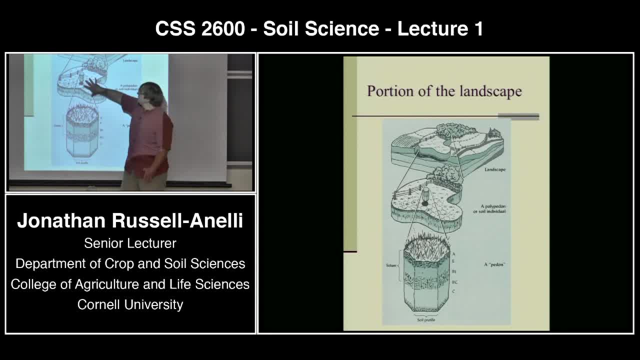 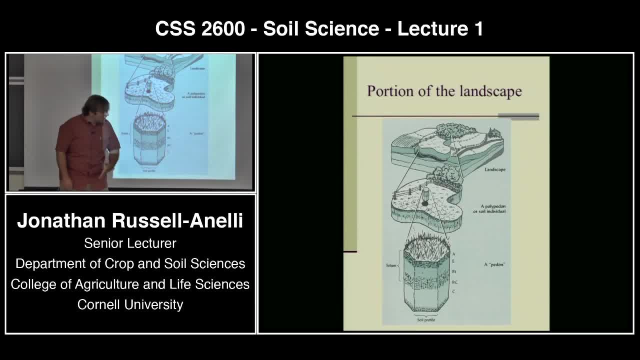 Okay. Okay, It's not necessarily true to what we see in the world. Sometimes it is discreet, Sometimes it's a very abrupt change, but often it is an attenuated change of properties across a larger landscape, And that's one of the big things that we're going to be talking about and learning about. 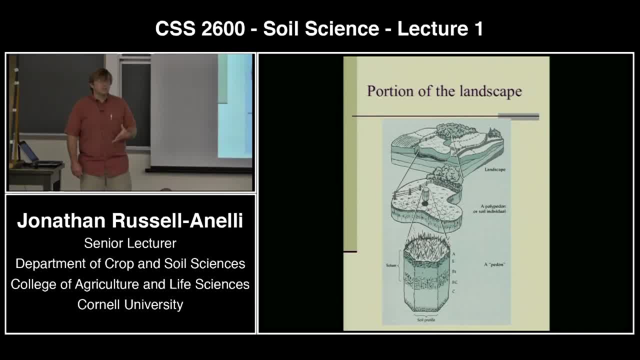 this semester. If you're a farmer, it's all well and good. It would be awesome if everything was very discreet. But if I'm growing corn on this side and corn on that side and I have two different soils but the attenuation between the soils is discreet. 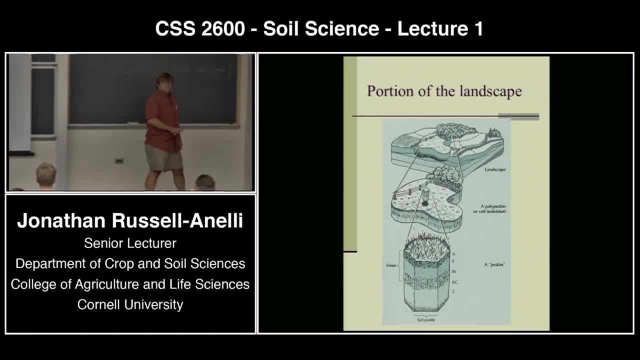 is very gradual. it's going to make it a lot harder for me to manage the corn on this side than the corn on that side. Does that make sense? And it's not just the farmer. What happens if I'm a homeowner and my septic system runs right through both of these? These are 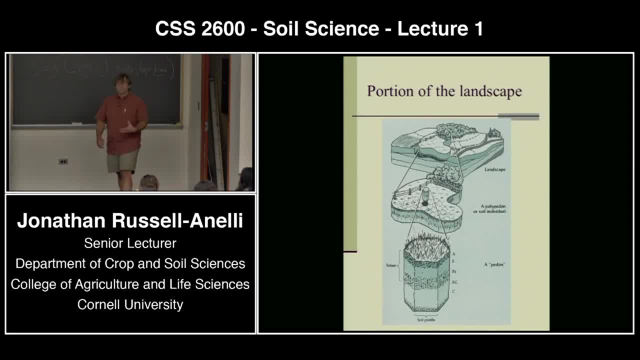 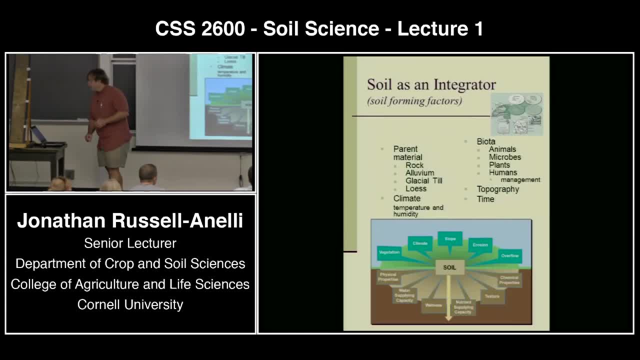 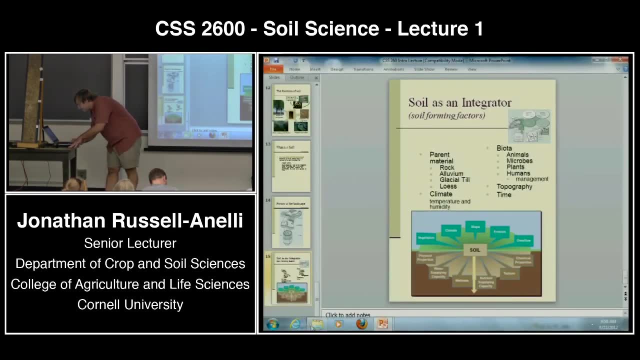 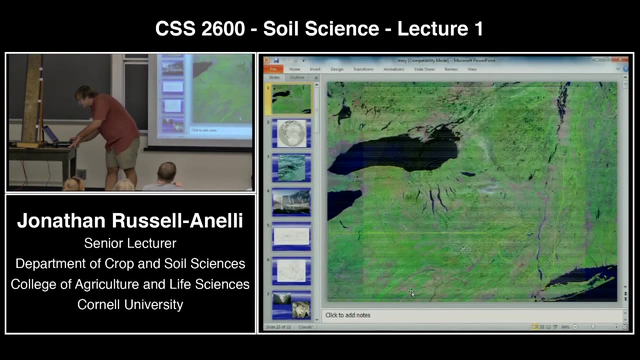 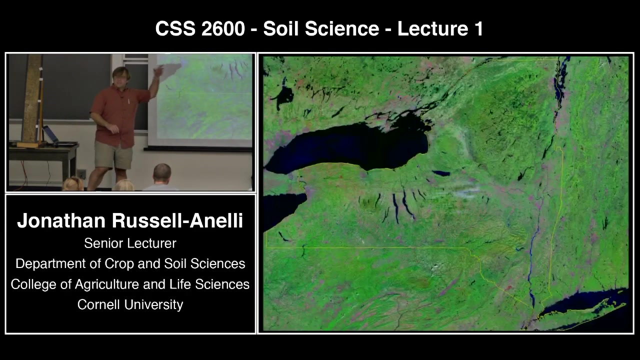 some of the things that we this is why we want to talk about this. Okay, Questions so far. We good to go on this. Cool, Let's go skip that slide And let's go to this. Okay, everybody recognize this. 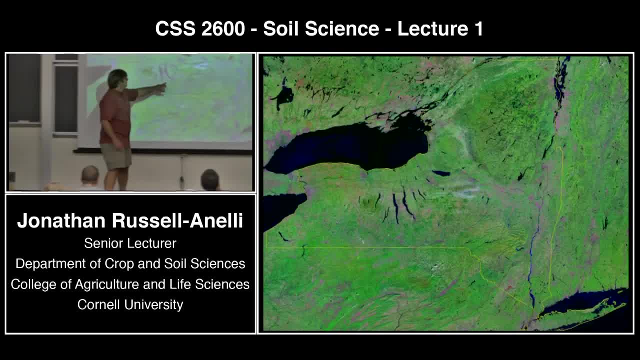 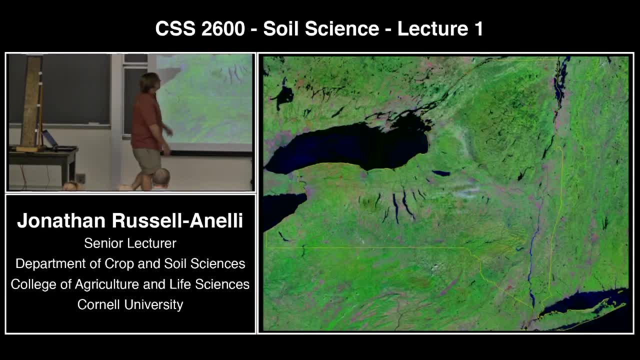 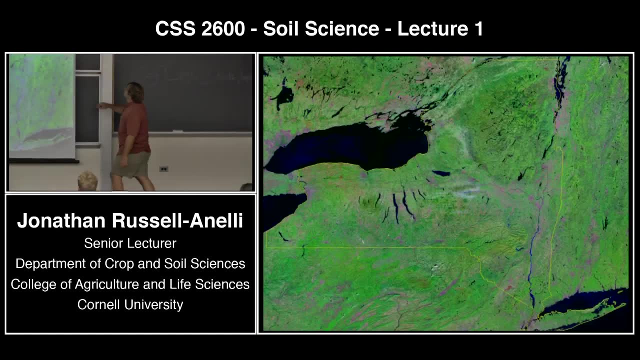 Over. Lovely. All right, You are here. Okay, this is the Finger Lakes. Okay, you got chunks of Ontario, a little squiggly part of Quebec, Pennsylvania, Connecticut and Vermont. Maybe a little bit of New Hampshire too. Actually, I guess this is probably New Hampshire border. 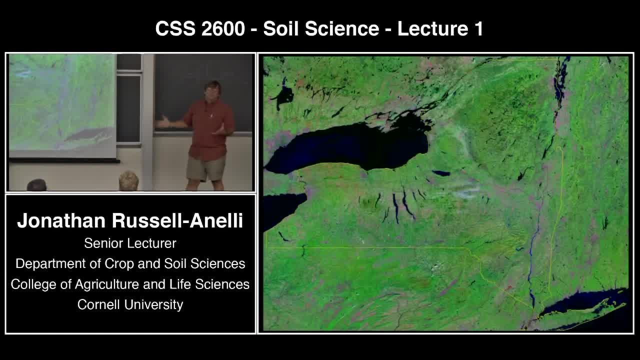 right there. Okay, This is the landscape that we're going to be operating in. This is not the landscape of the world, but it's the landscape of the Finger Lakes. Okay, And this is where I can drive you in essence. 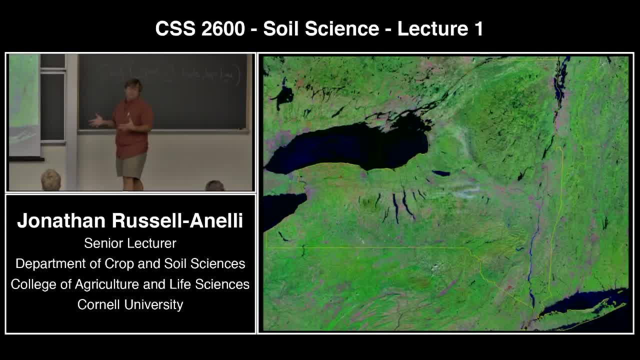 Okay, This is a landscape that is dominated by glacial history. Now you heard me say not too long ago that the soils around here at most are 12,000 years old. Okay, If you get down to about here, you're looking at 23,000 years, And if you're up there, you're. 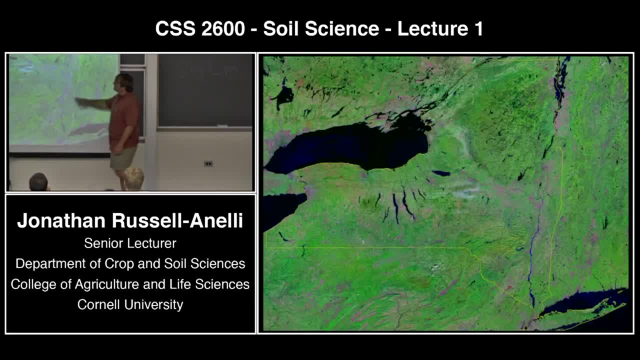 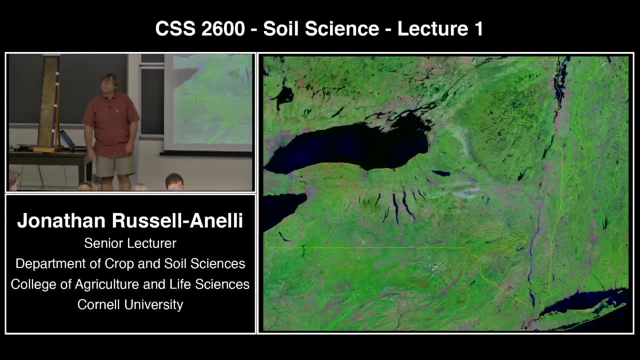 looking at about seven, eight, Okay, But around here about 23,000.. Well, why No, not 23,, 15,, 12,, 15.. Why? Well, that was when the glaciers came into existence. Why? Because they were. 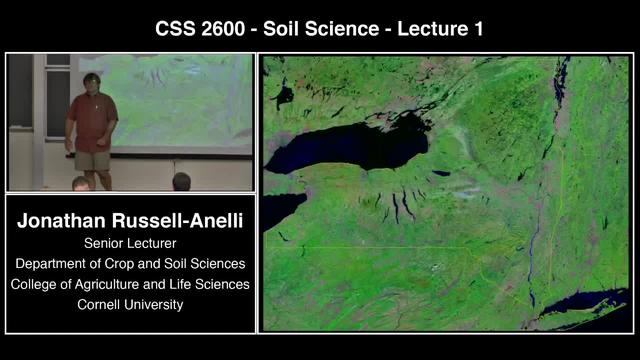 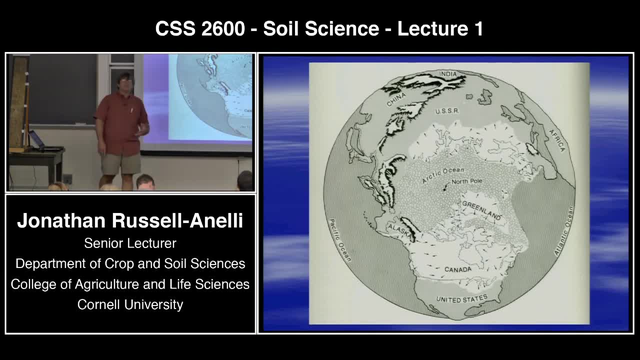 the glaciers finally receded from this region, Okay, About- well, there's actually a series of four of them, but about 250,000 years ago we had an advance in the glacier period, Okay, And basically the glaciers expanded from sort of the plate area of Canada between 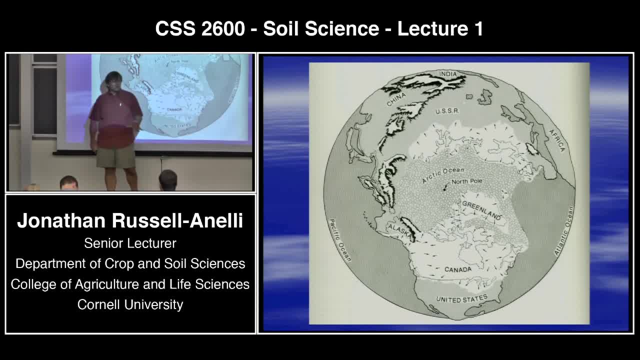 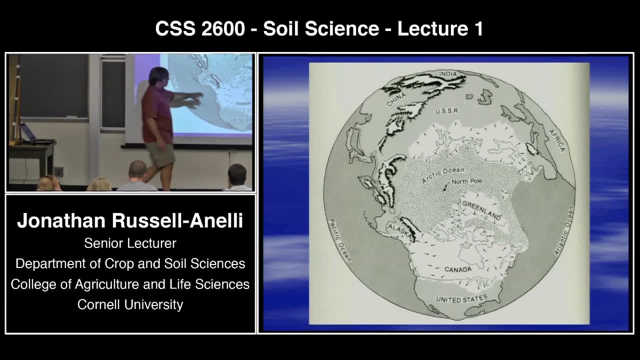 Canada and Greenland and sort of pushed its way down. Now does everybody know what a glacier is? I'll talk a little bit about what glaciers are, But basically glaciers are ice sheets that we have an accumulation of. Okay, And then you know, the glaciers are ice sheets that we have an accumulation of. 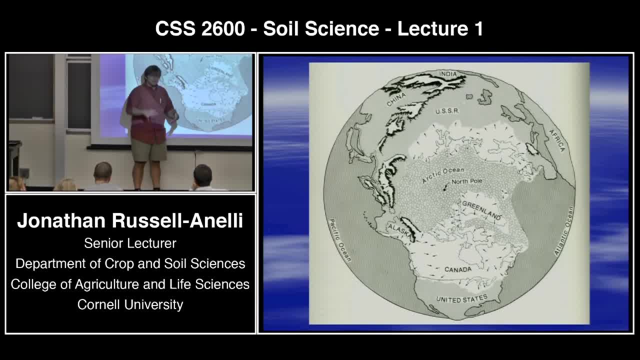 snow up here, which compacts. That compaction basically turns into ice, And if you have enough compaction, what's going to happen is it keeps pushing down and it will start to expand. Okay, And basically what you're seeing here is that expansion. Okay, It was. 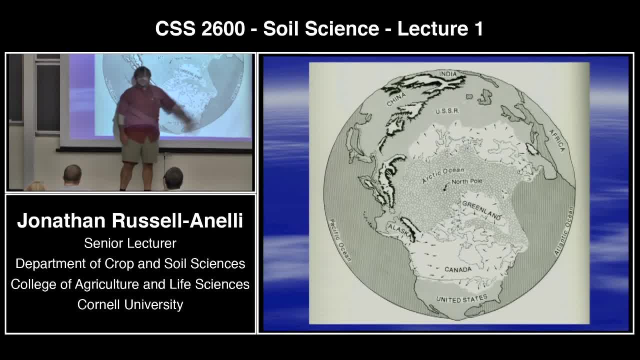 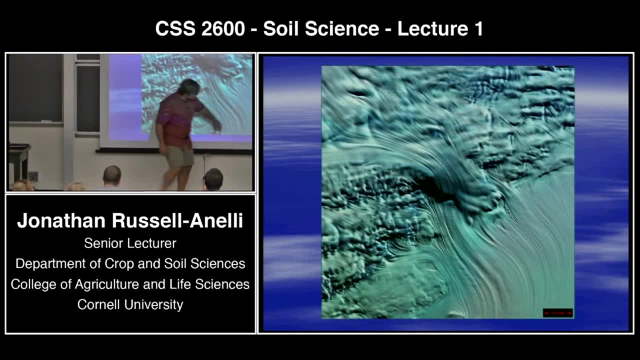 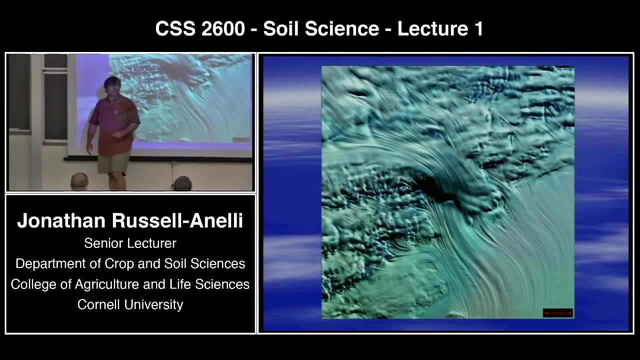 a very large event all the way up and across the entire northern hemisphere. Okay, And this stuff flowed. Okay, This is- I don't know if you can see this, but that's 4.4 miles. Okay, Basically, what you're looking at is the flow path of a glacier. It looks very much. 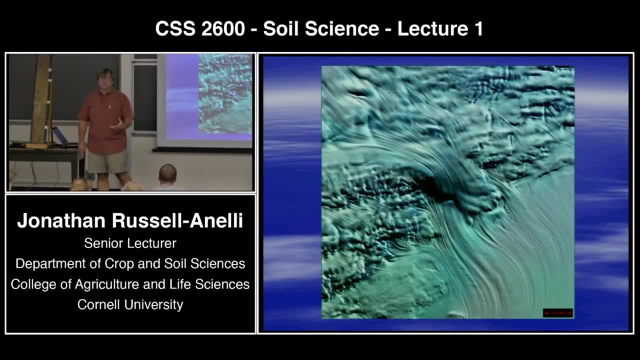 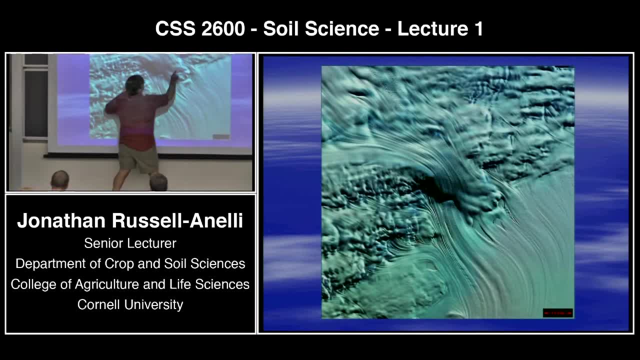 like water. In fact, it is water. It's ice, Okay. It just flows a lot slower than liquid water. Okay, What you can see right here is a ridge and a ridge with a glacier being forced right through the middle. You can see these two spots here. There's a third one. 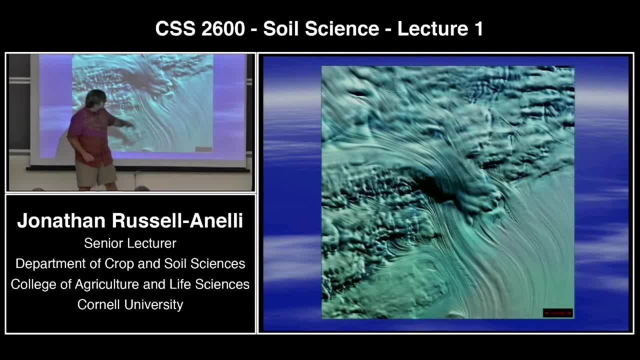 here And those are basically ridges. These are ridges coming up into the middle of it, So you can see a disturbance in the flow path, But you can see the flow path comes back and and joins up again. Okay, Now this is flowing by pressure coming from up here pushing it. 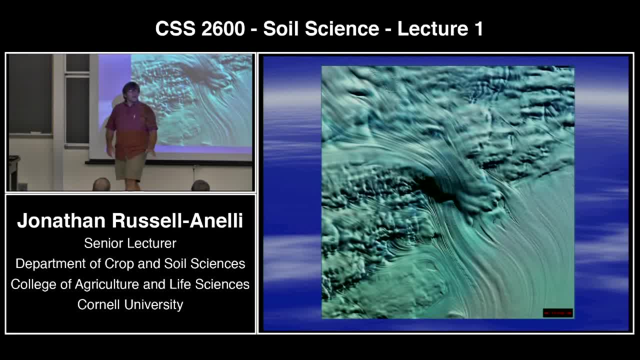 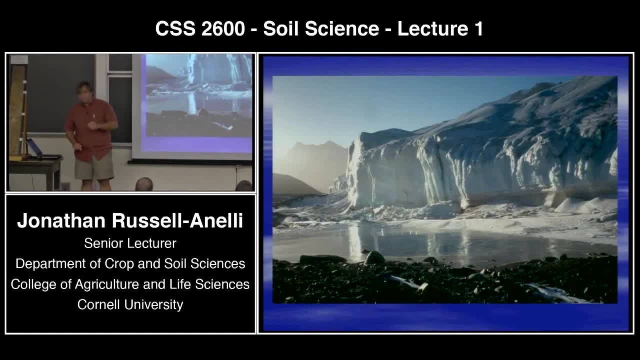 this way, Okay, And it's going to act like water, and everything that's in its path is going to get pushed. Some of it's going to get scraped, but it's going to get pushed forward. This is what a leading edge looks like, except this is a receding leading edge. 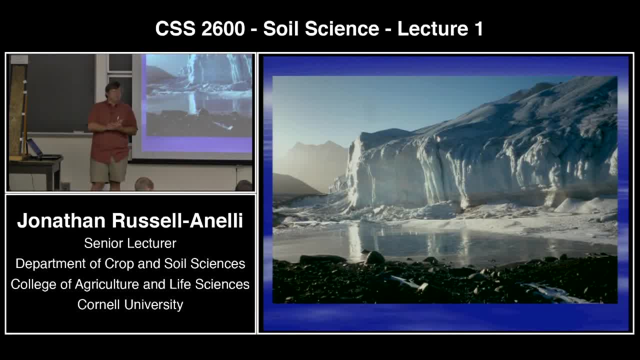 We don't have. I'm not sure if this is quite true. I don't know of any. I don't know if this is a receding leading edge. I'm not sure if this is quite true. I don't know of any. 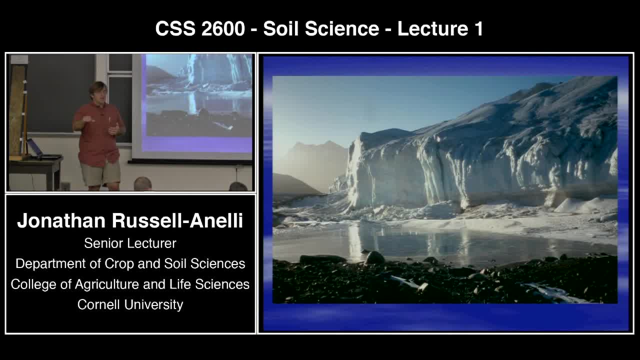 I don't know if this is a receding leading edge. I don't know if this is a receding leading edge. We're still seeing glaciers that are pushing forward at a rate that we're seeing dramatic accumulations in front of it. They are still moving forward, but in general, 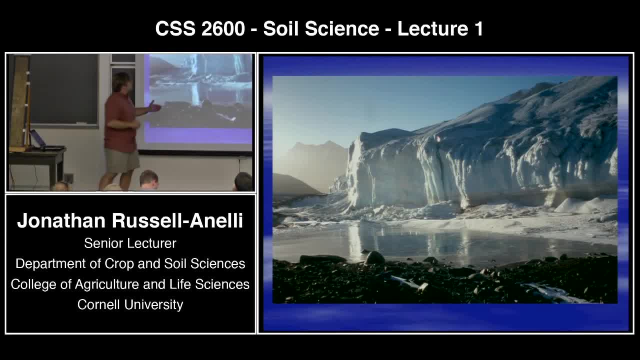 they're all receding because of global warming. Okay, But basically what you see is a front edge that looks something like this: You see this debris field in front of it. This debris field at one time was probably where the ice was, And the ice is probably way rigged that. 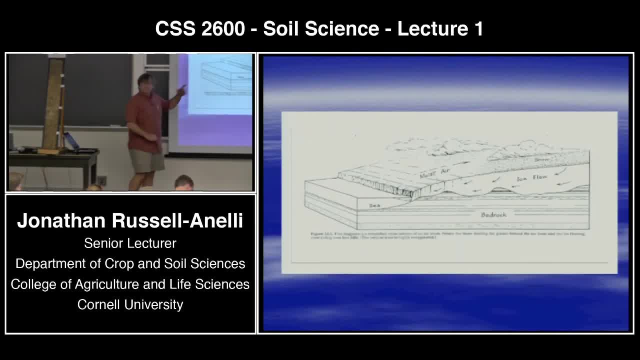 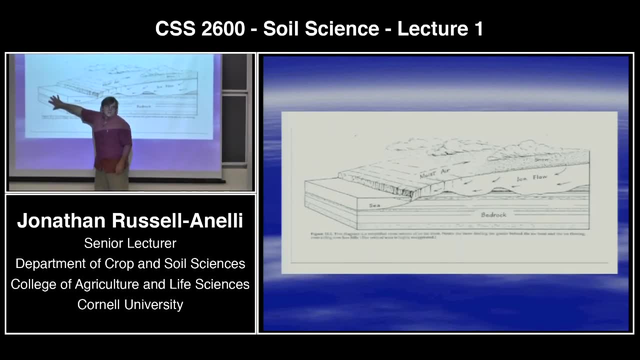 way? Okay, How this works. can you see this slide? Does this slide all right? Can everybody see it in the back? Okay, this is basically a graphic to show you how these flows work. So imagine the ocean, a warm body down here, with water down here. okay, higher elevation up here. 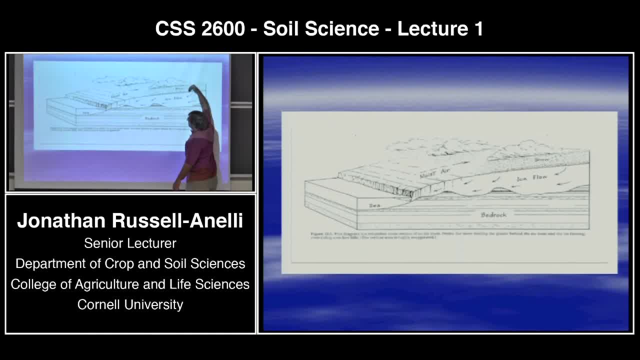 What happens is you've got cold air coming through this way and pushing through this way. okay, It hits the sea. warm evaporation, evapotranspiration- that water gets uplifted and then gets sucked into moist air up to the top of this landform and gets deposited as snow. 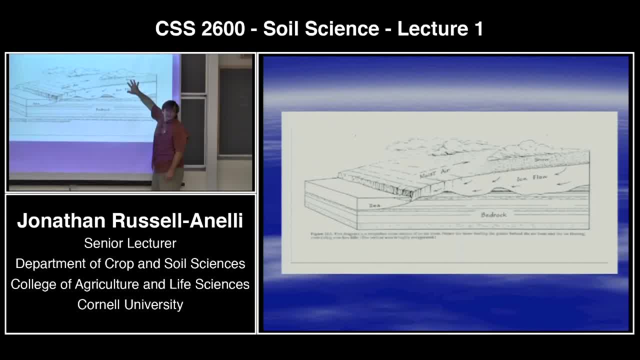 Make sense. Okay, the snow accumulates and accumulates, and accumulates and ultimately you start having ice flow. The ice basically flows over the landscape below it and, as it flows over, there's a number of different ways why it flows and how it flows, and we'll talk about those. 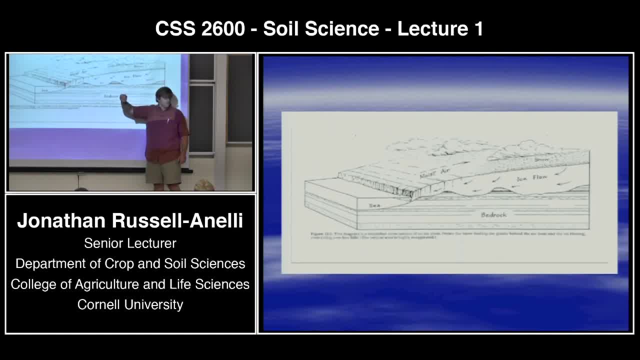 but as it flows over, it carves out the landscape below it. Does that make sense? Okay, now this will keep pushing. It's going farther, farther, farther, towards the warmer zone, until the point is reached at which it melts as fast as it grows. 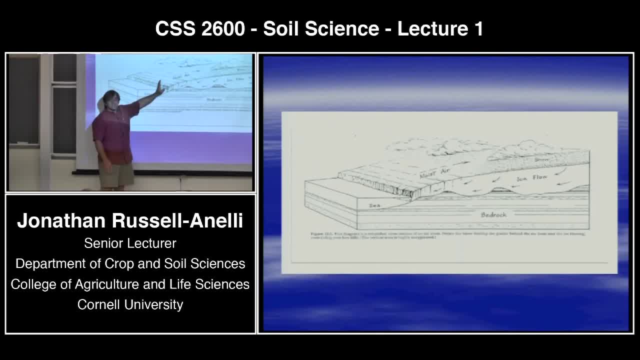 Okay, does that make sense? We call that point basically a dynamic equilibrium, where the ice is advancing as fast as it is melting. Okay, sooner or later, all things being equal, sooner or later this system is going to stall, for whatever reason. 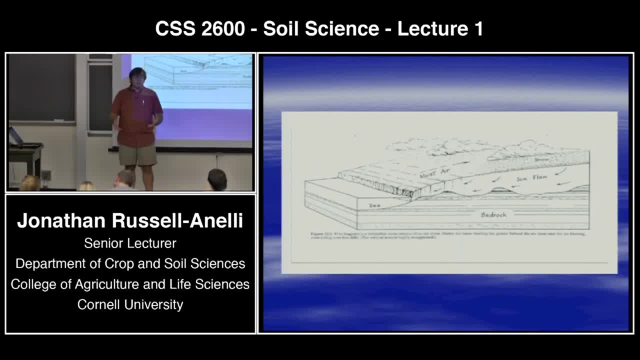 The temperate. the climate might get warmer, which it is right now, or you might have less moisture coming into the system, or you might run out of the water. Okay, sooner or later, this glacier is not going to advance anymore. 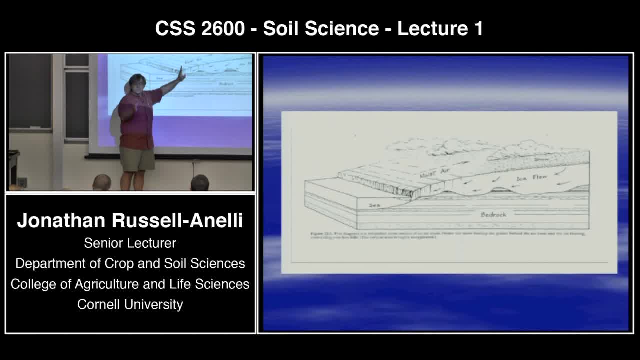 at which point it's going to be, at that stable, that dynamic equilibrium. Now, if anything changes, this glacier is going to restart receding Now. receding is probably a bad word for this, but it's the common usage. It's not like the glacier, like a rubber band, where it starts retreating. 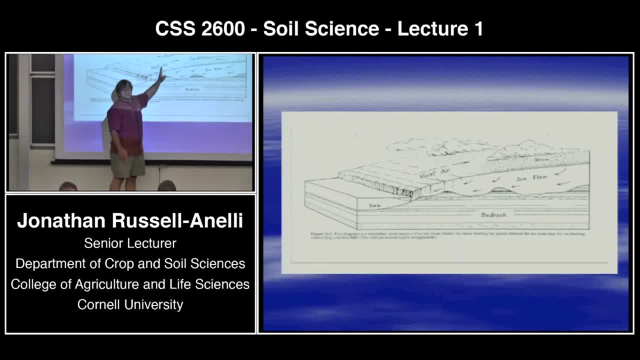 What's happening is really is: the front end is just melting and it looks like it's retreating. Okay, and if it's melting, everything that is in that ice up to that point basically gets deposited there. Okay, now, as it was pushing forward, it was pushing a whole load of stuff in front of it. 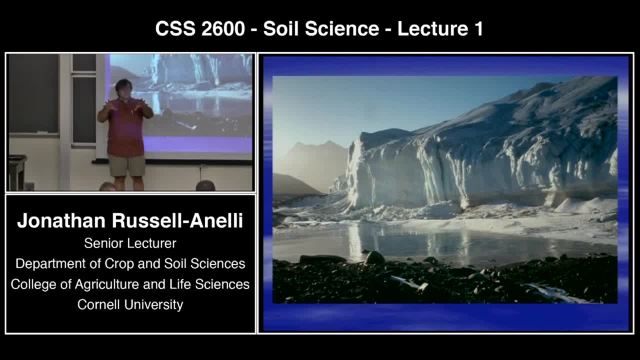 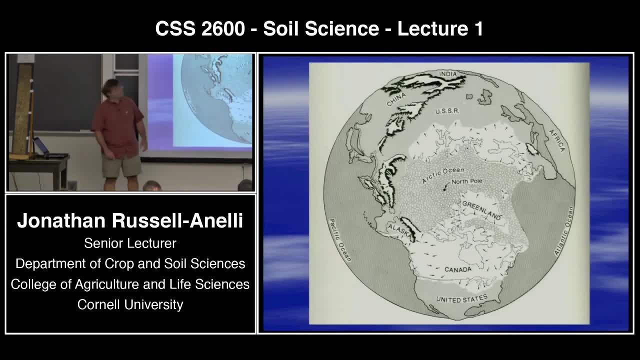 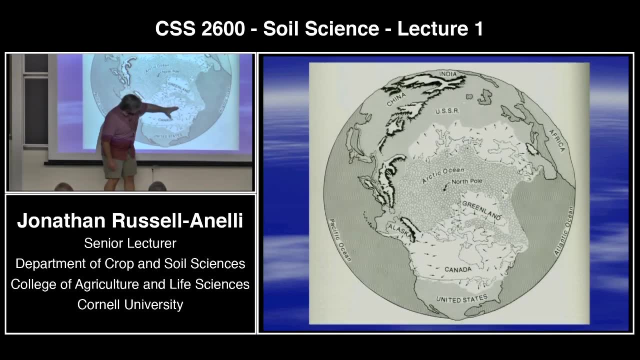 All this stuff is being pushed, Okay, And it has been carried by the ice for a long distance. I mean, you saw how large this expanse was, So some of the stuff that we're seeing down here, because this ice basically started up here. 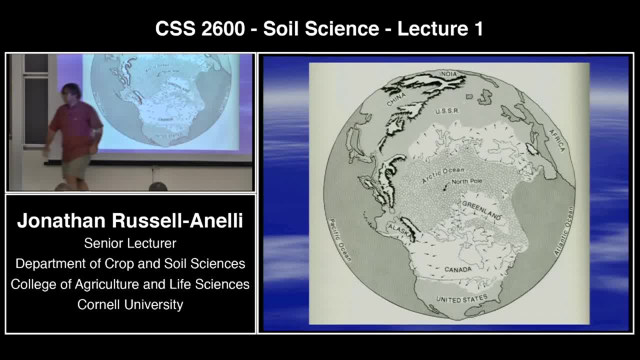 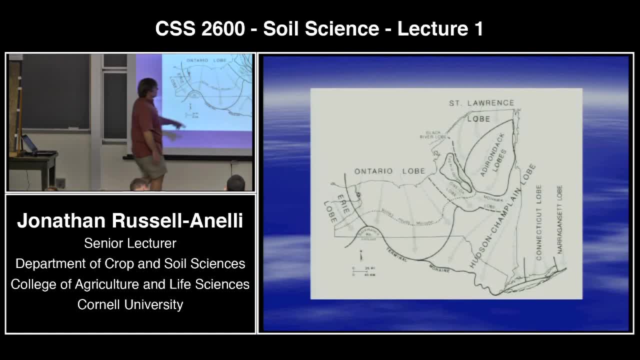 literally came from up here and is deposited. All right, so let's come back to the Finger Lakes. You are here or thereabouts. Okay, this is the Ontario Lobe of the Wisconsin or the Wisconsin Glacial Epoch. This lobe basically drove through central New York. 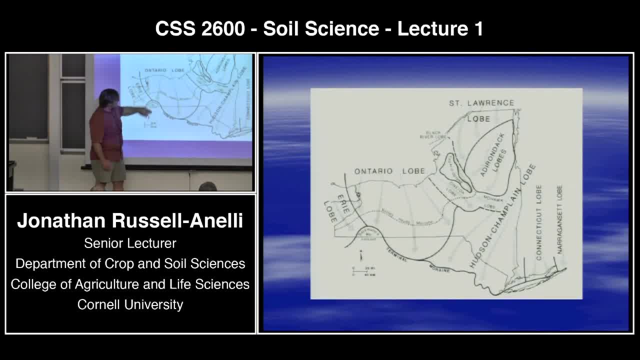 and came down to northern Pennsylvania with one little section right here that's called the Salamalca Retrenchment. This is the only part of New York State that was not under the last glacial period. That's not to say that it wasn't under glaciers. 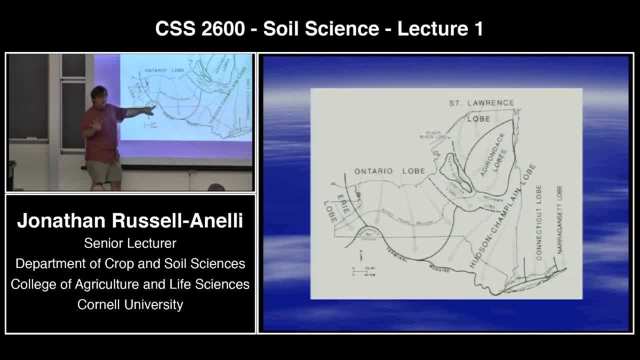 The Wisconsin. the last glacier was the fourth of known glacial events. Okay, now, this was. This was also combined with a montane, a mountain glacier, which was the Adirondacks. This was not a continental glacier, This was a mountain glacier. 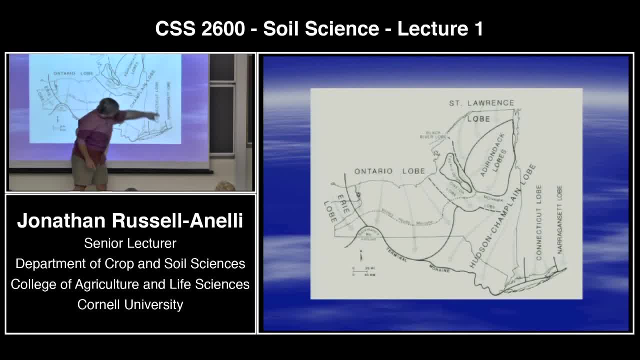 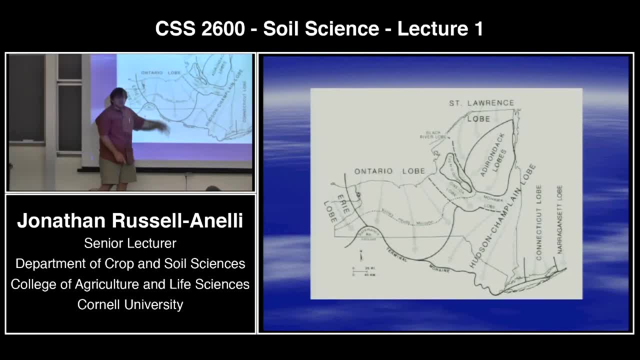 Okay, They combined to basically push the glacier front down to this line right here. So basically all of New York, except for this one spot here, is glacierly formed, or modified, maybe the better word. Okay, Okay, Long Island Turns out to be basically two rock piles. 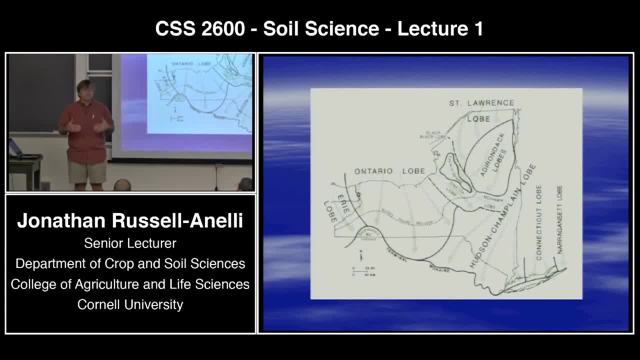 that were pushed up and dropped in front of the glacier. It is the pile of material that the glacier pushed up. Now, if anybody's from Long Island, you know how large Long Island is. And even if you aren't from Long Island, 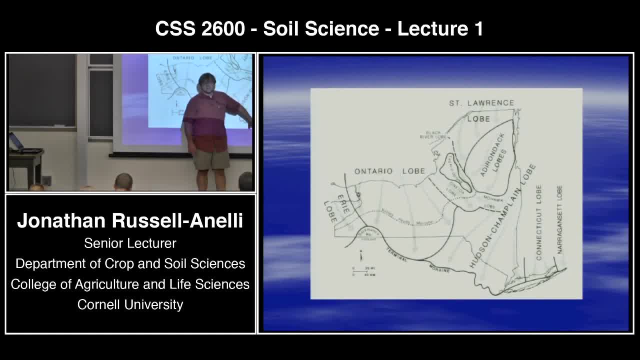 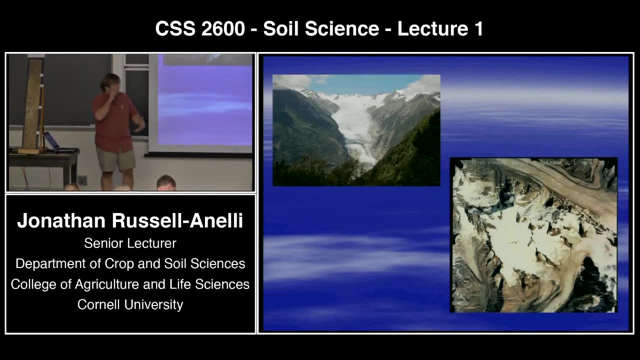 I mean, look how large that island is. That island is formed from a debris field pushed by ice. That's how big this was. Now I also mentioned that we had these montane glaciers, the Adirondacks. These are glaciers that basically form on the top of mountains and then flow out of it. 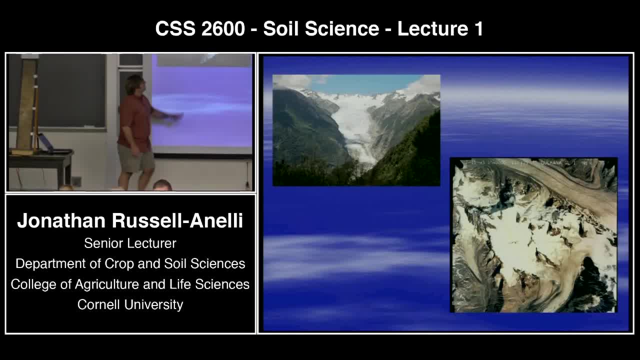 Okay, Here is one where you're looking up at it, but you can see that this valley is very sort of U-shaped, being pushed down because of the ice. This is called the Cirque Valley. The ice goes down, I mean just like water. it's going to flow downhill. 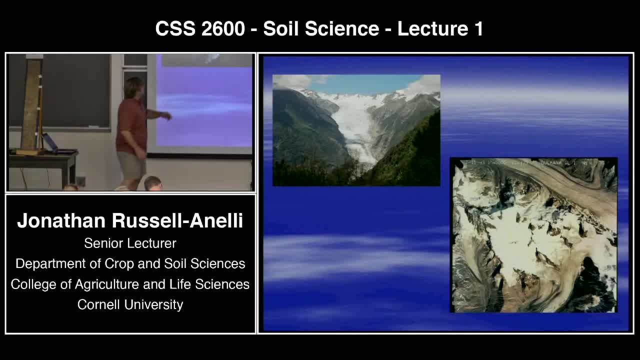 It's going to flow into those low spots and then push down and basically, as it pushes down, it carves out that landscape. Now this is important, especially for around here, because the same process- now this is not a montane glacier around here, but the same process that carved- 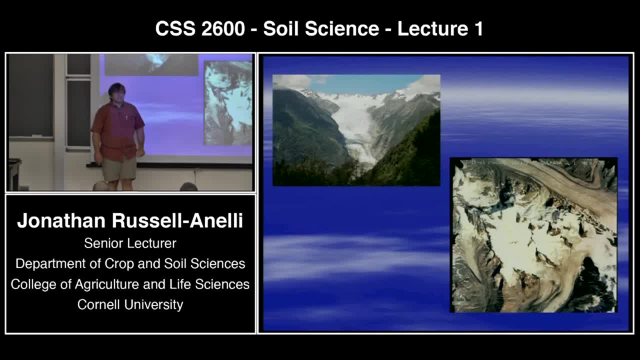 out this? U is the same process that carved out the Finger Lakes. Okay, And I think I am out of time, We will continue this story on Friday. I know some of you are going to miss it Again. before you guys go, check the website and if you are, 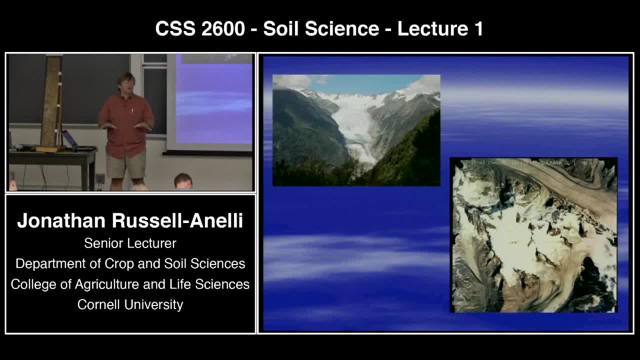 in the Monday lab and you have the option that you can move to Wednesday. please email me or come contact me, because we are over-enrolled in the Monday lab. Okay, All right, guys, Have fun.